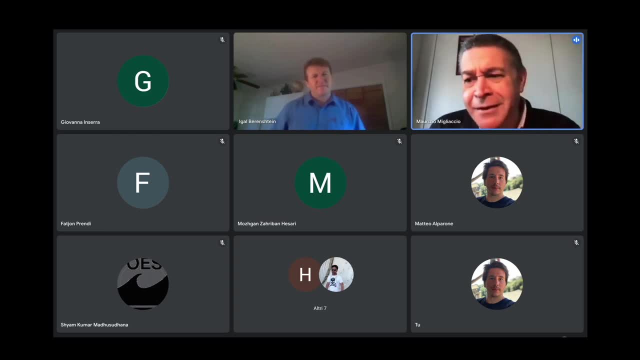 sensing guys. you have some and in that school there is even a center for remote sensing and but you have to even deal with the some delicate choice and just a premise to you, for example, how much and which kind of this person you may like to use, which are kind of. 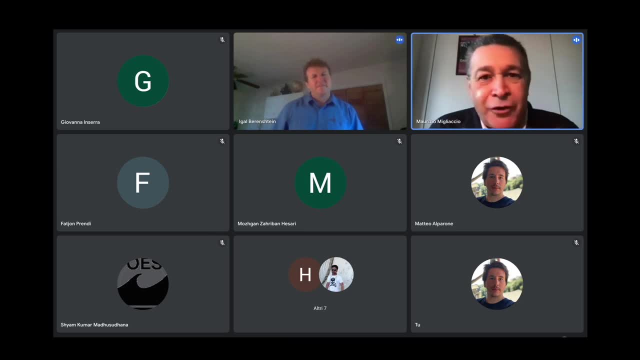 something, let me say, chemical, that breaks the, the film of oil but is not uh so healthy for the environment. so it's kind of balanced and of course, for this it's very important the, the in the team, let me say that you have the ecologists and so on, and today, uh, i give you the words. we have the. 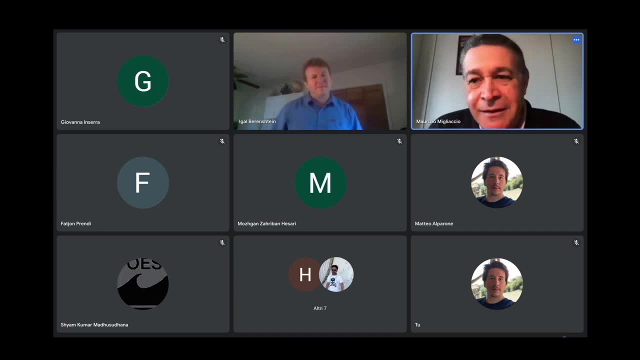 the, the the pleasure and the honor to have eagle berenstein discussing about the gulf of mexico oil field accident, which was a challenging uh test. we hope to don't have many other times, but it's still a material investigation after so many years, both on the remote sensing side. 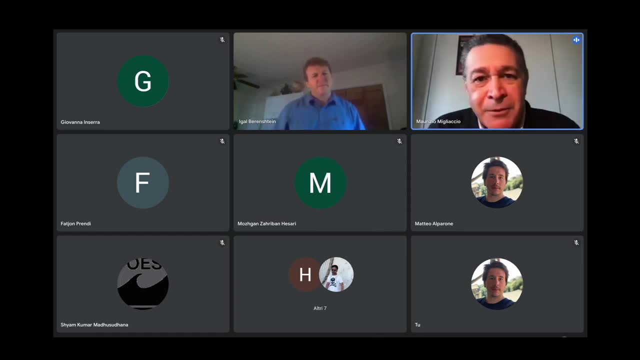 on the ecological side. there was very famous paper about valentine on. you know long-term effects, okay. so it's like a, a, a very, very important experiment, let me say, with respect to the, the positrons of the agriculture, when we contain so many of the, the clinics of montanes and the uh that enter there, for example during the ex jam練 section. 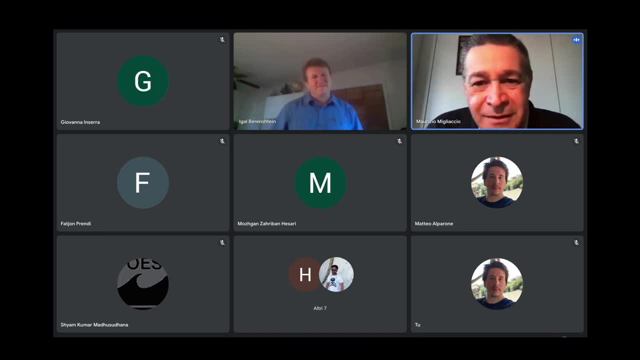 and the fact that the visceral explicar press is driving this Latin social process and therefore, as you can see, the couple problem at one place is all, mr, not changing the place it choose to be at another point, but nonetheless we will let, that being said, how you exit me hope. Всем vielen Dank. 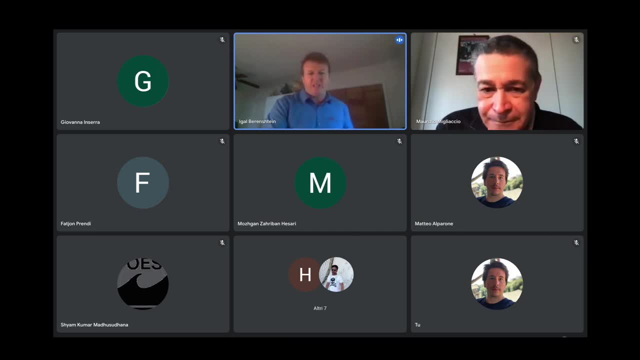 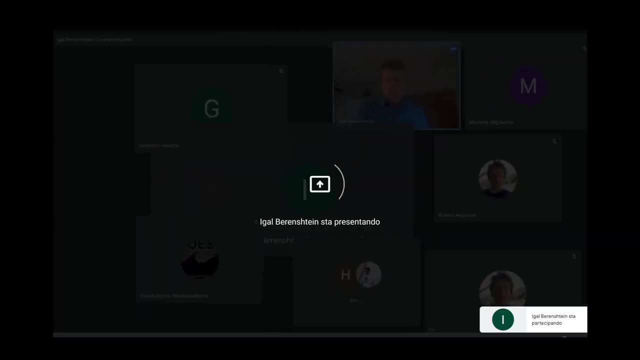 have to understand for future accident. we hope happens, but you never know, and uh, i i don't want to wasting more time and i keep the word to eagle, berenstein, Panda, Art of mirroring lice in to start this seminar. thank you very much. talk a little bit about that in my presentation. let's see just that you can. 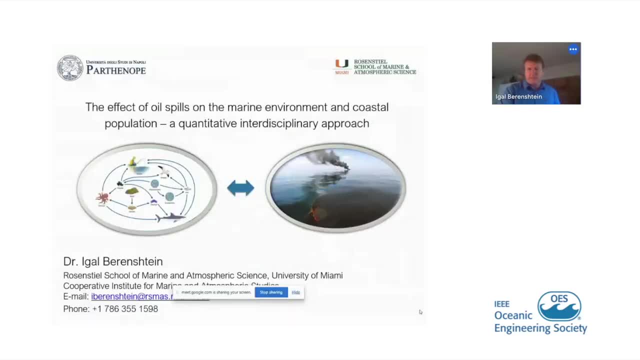 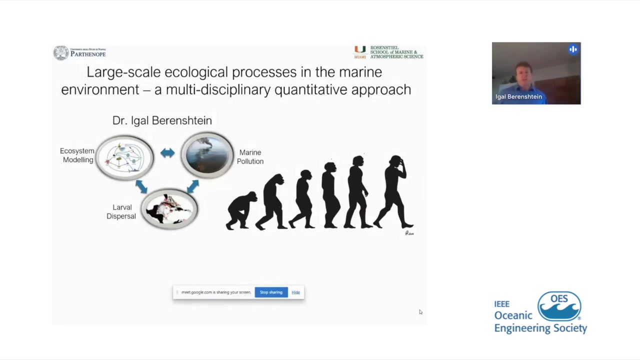 see my screen. can everybody see my screen? yes, okay, perfect, yes, so yeah, today I will talk about the effect of oil spills on the marine environment and on coastal population using a quantitative, interdisciplinary approach. so just a brief history of what I've been doing and where I come from. so I did my PhD. 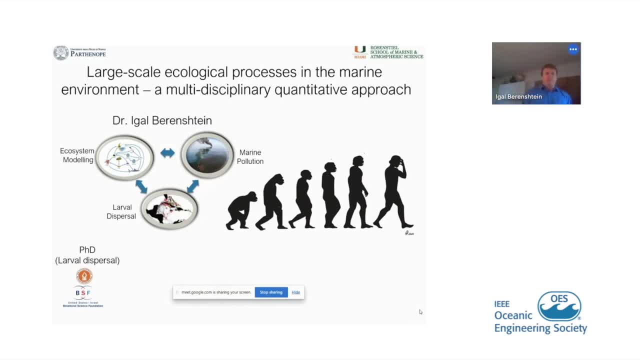 working on larval dispersal and connectivity, biophysical modeling, larval orientation, and from there that was in Israel, in Ben Gurion University. from there I went on to Israel in Ben Gurion University. from there I went on to Israel in Ben Gurion University. from there I went on to work on marine pollution during my 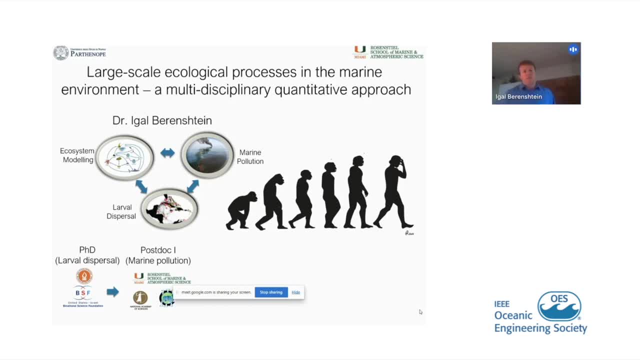 to work on marine pollution during my to work on marine pollution during my first postdoc at the Rosenstiel School of first postdoc at the Rosenstiel School of first postdoc at the Rosenstiel School of marine atmospheric science in Miami. after that I moved on to work on: 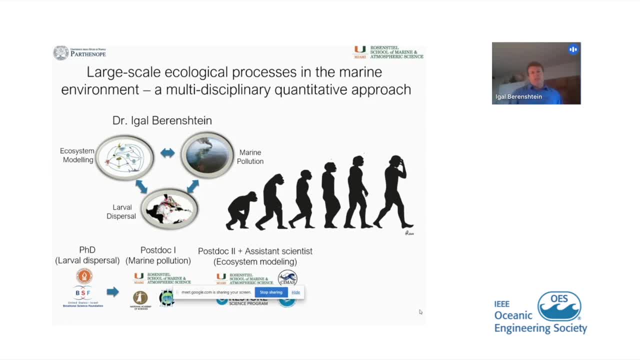 after that I moved on to work on. after that I moved on to work on ecosystem modeling in the Gulf of ecosystem modeling in the Gulf of ecosystem modeling in the Gulf of Mexico during my second postdoc and Mexico during my second postdoc and Mexico during my second postdoc and assistant scientist position and next. 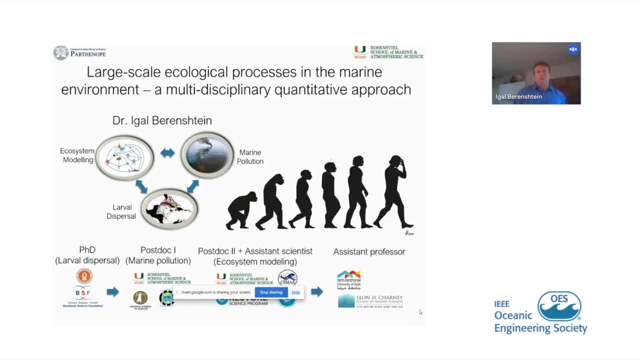 assistant scientist position and next assistant scientist position, and next year I will start a position as an year. I will start a position as an year. I will start a position as an assistant professor at the University of assistant professor at the University of Haifa in Israel, and in this talk today, I will focus on the work done during my first postdoc. 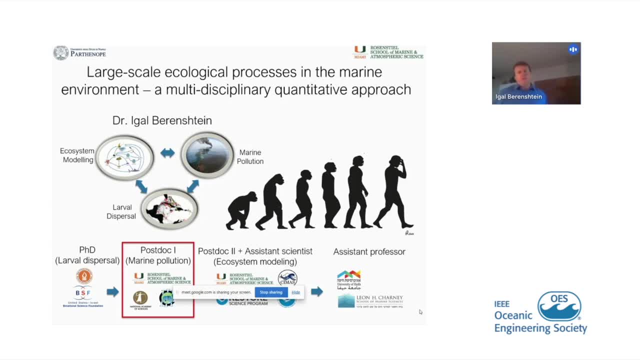 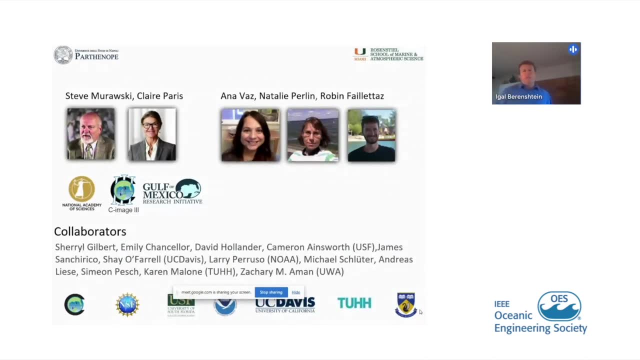 working on marine pollution, primarily in the Gulf of Mexico, and I will first want to acknowledge some key personnel, key people in that in this work. so Claire Paris was my first postdoc advisor and a mentor, and in her lab the oil CMS, oil transport and fate model was developed. 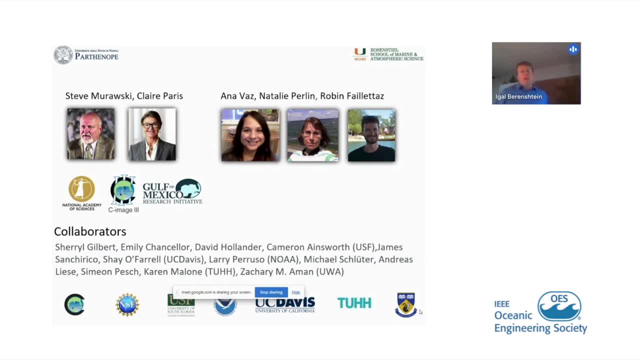 and she is a PI on two main funded projects funded by the National Academy of Sciences and the Sea Image 3 Consortium, which is under the umbrella of the Gulf of Mexico Research Initiative. and also I want to acknowledge Steve Murawski, who is the main PI of both of these projects and as well as a scientist from Claire. 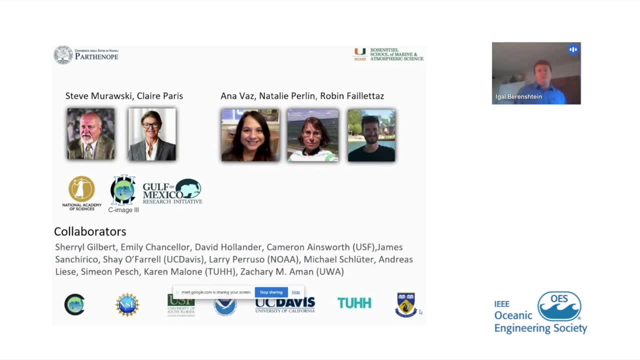 Paris's lab, Anna Vaz, Natalie Perlin and Robin Filetas, who worked on developing the oil CMS model and the products associated with it. I would also like to acknowledge various collaborators that contributed to the to the development of the model and the associated projects from various institutes in the US and in Europe and in West Australia. 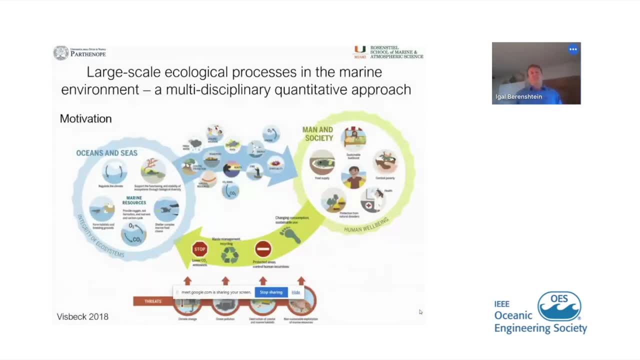 and so why is it important to study large-scale ecological processes in the marine environment? so our life, as we know it is completely dependent on the unhealthy oceans for clean air, for a drinking water. through desalination, the oceans regulate our temperature, the the temperature it takes in carbon dioxide. 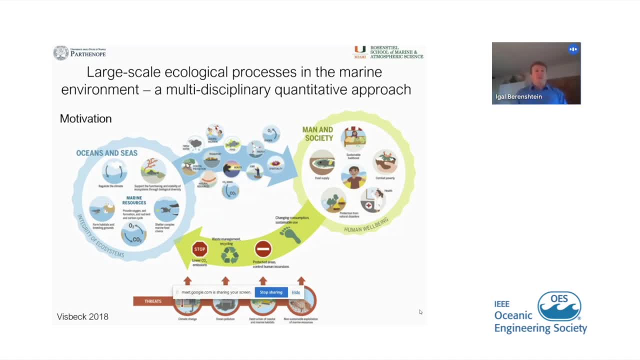 it includes hundreds of thousands of marine species and it provides a livelihood and nutrition to millions of people in coastal uh population around the world. but this important asset, this critical asset, which once seemed infinite, is quickly deteriorating due to marine pollution, due to climate change and overfishing and in this 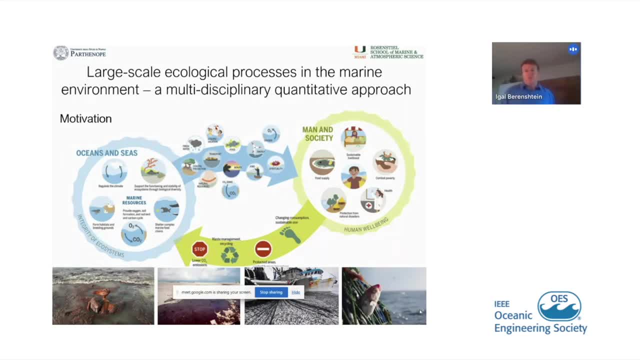 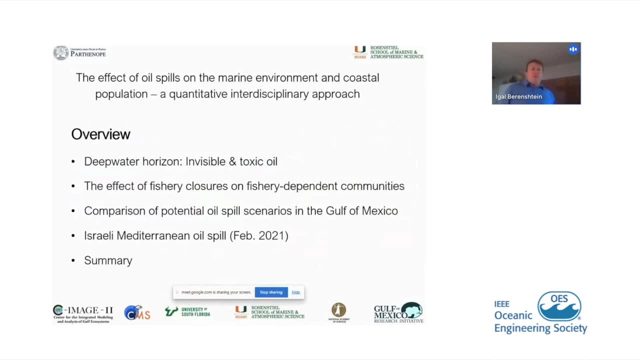 talk, I will focus on the aspect of marine pollution, and so I will give you a brief overview of the talk. I will first talk about the deepwater rising oil spill and the invisible and toxic oil that we found was part of the spill. I will then talk about the effect of fishery closures. 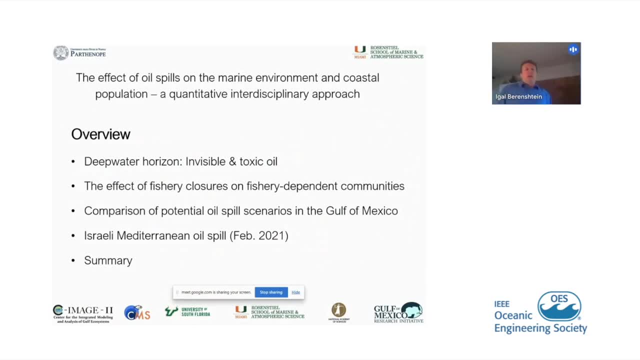 on fishery dependent communities, and I will tell you about a computational framework that is able to compare potential oil spill scenarios in the Gulf of Mexico, and I will briefly talk about the Israeli oil spill that occurred a year ago go. I will then summarize and conclude the talk. And so during my first postdoc, I worked. 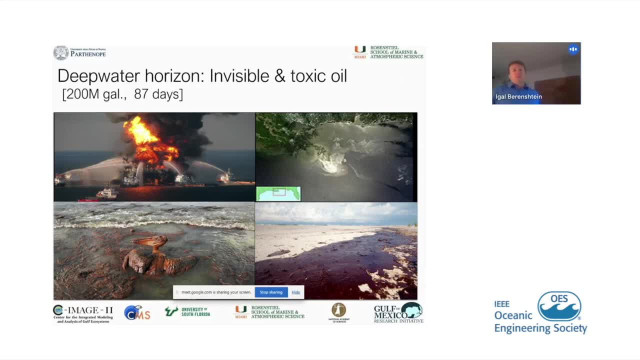 on the Deepwater Horizon oil spill. It was one of the largest marine oil spills globally. It released more than 200 million gallons of crude oil to the Gulf of Mexico. It lasted for more than 87 days. It contaminated vast areas of the Gulf of Mexico, killing an enormous 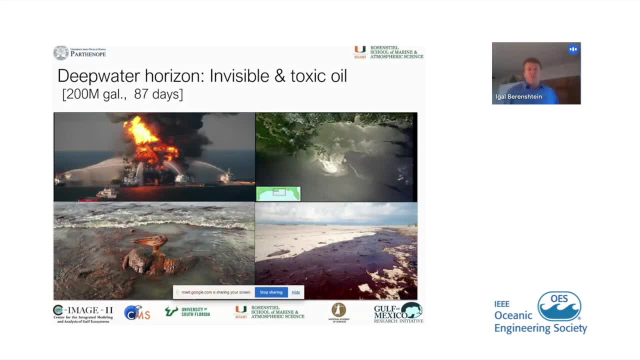 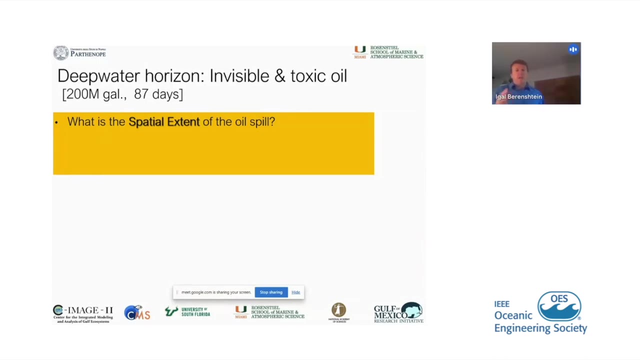 amount of marine wildlife- fish, invertebrates, marine mammals. It harmed coastal habitats and, even to this day, some of these areas are closed due to this spill, And so, as a marine ecologist, my first question when starting to work on this oil spill was: 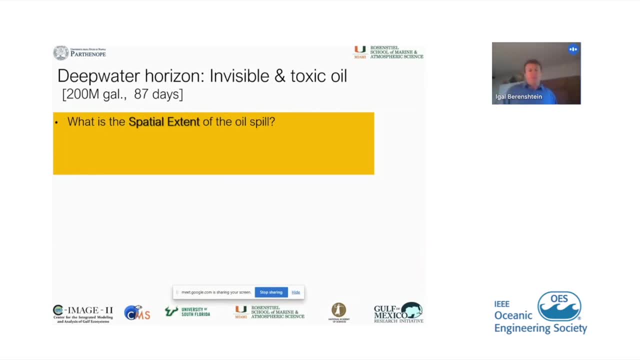 what was the spatial extent of this spill? And when I asked this question, the answer I kept receiving: is the satellite footprint detected by satellites, or visually or from planes, and this was considered the spatial extent of the spill. And so then I asked: does the satellite footprint, or what was visually identified, accounts? 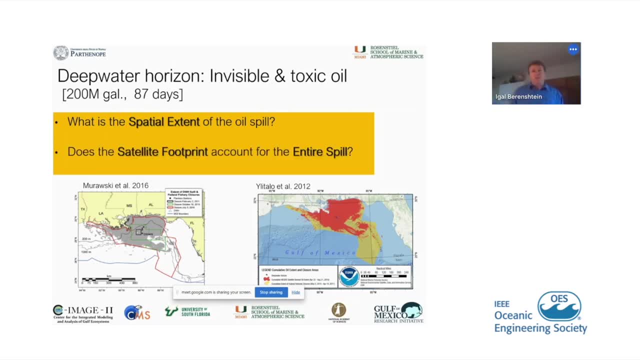 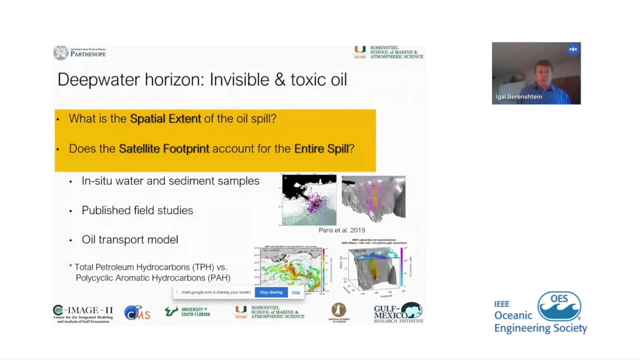 for the entire oil spill, And to answer this question I used three main sources of information: More than 40,000 in situ water and sediment samples, independent published field studies that examined the occurrence of oil in the Gulf of Mexico, and an oil transport and fate model developed. 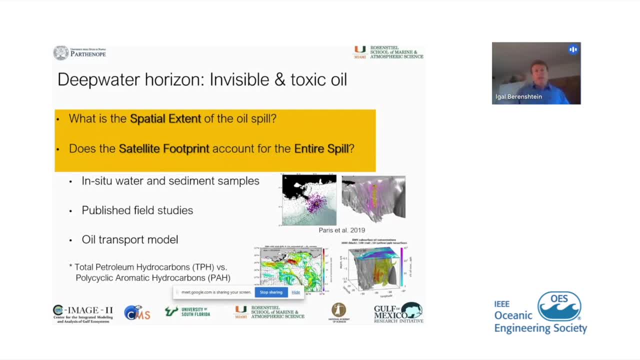 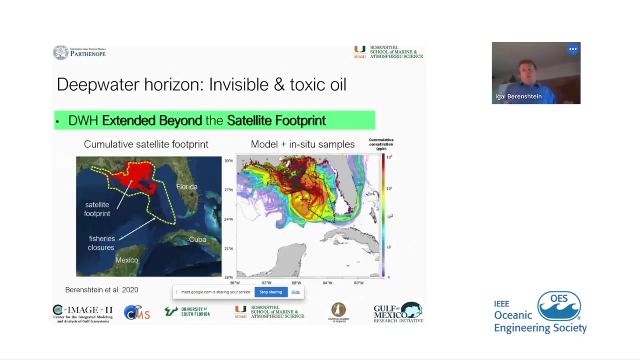 in the Claire Perry's lab, And I will briefly define two types of concentration, which I will talk about: TPH, total petroleum hydrocarbons, which represents the crude oil, and the polycyclic aromatic hydrocarbon, PAH, which represents the fraction that is mostly associated with oil toxicity, And so what? 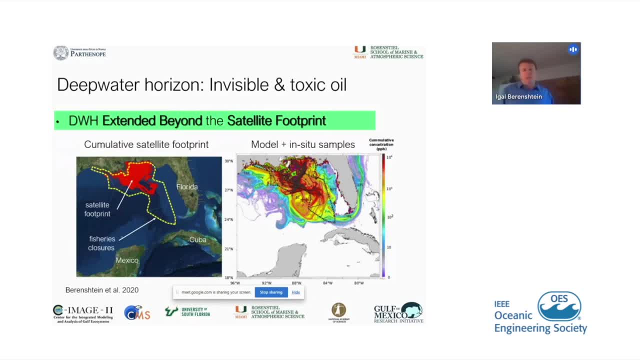 I'm going to do is ask the question: what is the spatial extent of the spill? And I will tell you more about it in a moment. And if we go to the left, you can see that the original location of the spill was in. 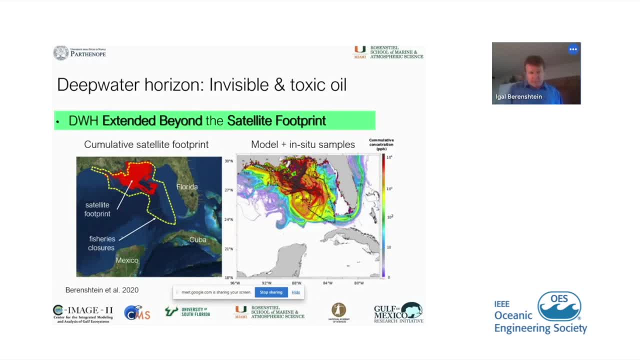 the lower right-hand side of the slide, And so what we see here is that the location of the spill was in the lower right-hand side and the location of the spill is in the lower left-hand side, And we can see the location of the spill. You can see the ground so from the left. in red color you can see the cumulative satellite footprint of the oil spill And what you see in yellow dashed line is the fishery closures that applied, based on the location of the spill detected by satellites and based on where they thought the oil would get to, And on the right-hand. 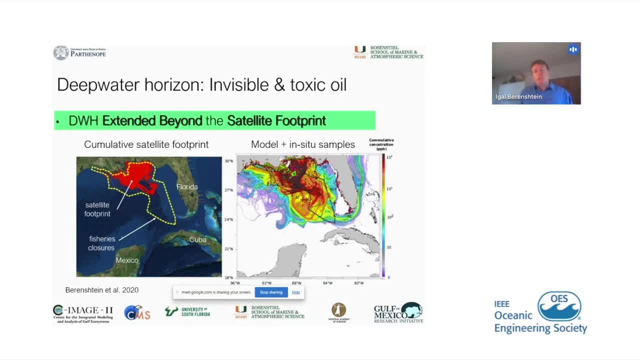 side you can see these three sources of information And the once you have the high ground information that i mentioned. so the different colors here are the results of the oil spill model, the oil transport model, um, and also a hot, like red colors, represents high concentrations and 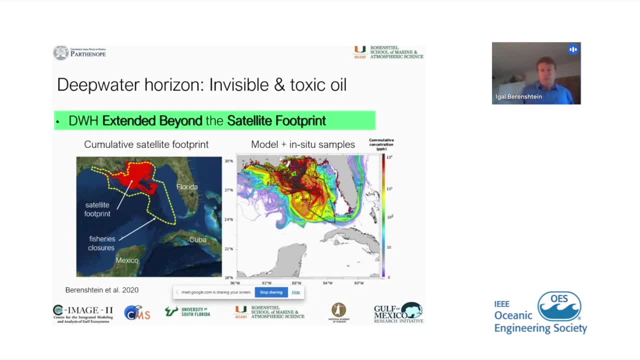 a blue and a purple colors represents low concentration. um, what you can see in a red as red dots are in situ water and sediment samples that were with concentrations above the the background level, and what you can see in red crosses are independent studies that indicated the presence of oil in these regions and what we can see clearly from these. 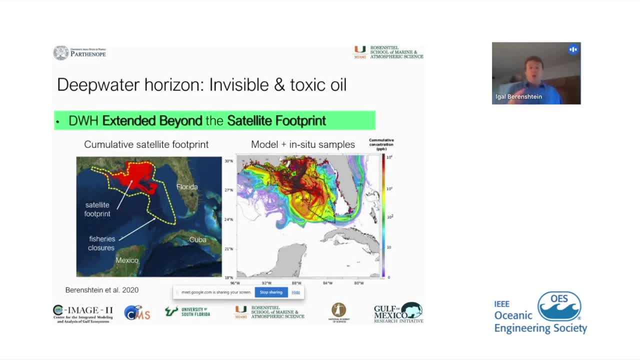 three types of information. is that the oil spill, according to these three types of uh informations, um exceeded beyond what was captured by the satellites and beyond the fishery closures. but then i ask: well, maybe it doesn't matter, i mean, if that portion that exceeded beyond the satellite. 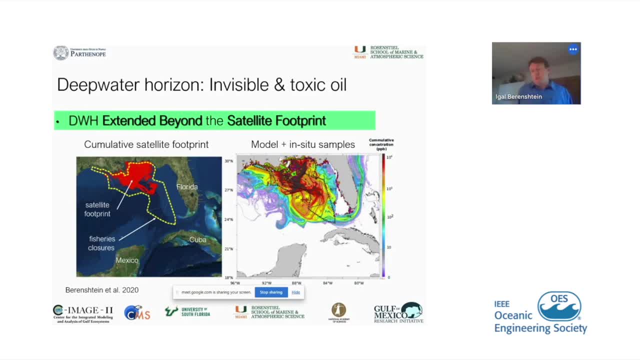 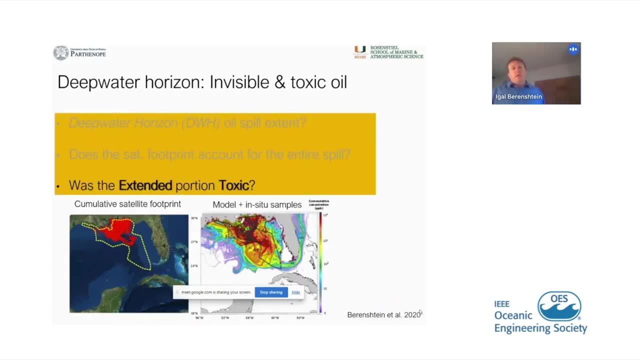 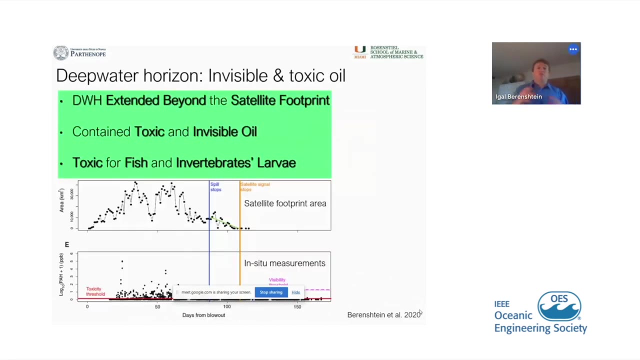 footprint and the fishery closures was not toxic to marine wildlife, then we should not care about it. so my next question was to ask: what was that extended portion toxic to marine life? and first i wanted to compute the satellite visibility threshold and basically what i did, what we did is to look at the time period for after. the satellites did not. 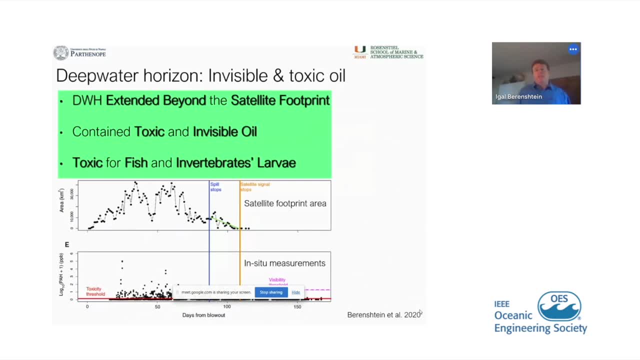 identified any uh oil slicks after the spill was cut. so what you see on the upper plot is the area detected by the satellite, the area of slicks detected by satellites, and what you see on the lower panel is the in-situ measurements that were measured. 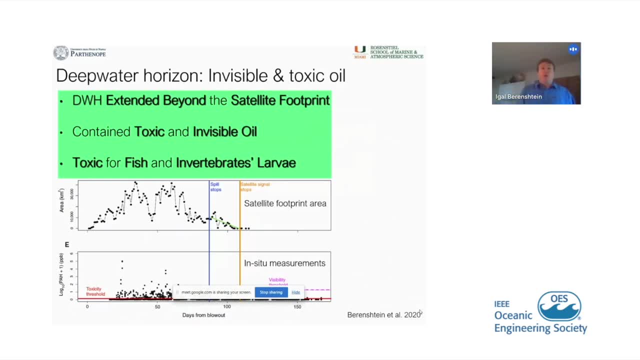 in the water during the spill and what we can see is that, after the spill was capped, there was a decline of the satellite footprint and then, at the certain point in time, there was no longer identification of oil slicks by the satellites. but at the same time, the in-situ measurements indicate that there were high concentrations of oil in these areas. 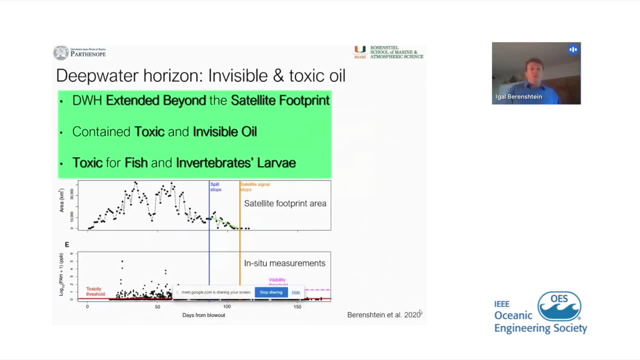 which are a higher, which are considerably higher than the toxicity threshold. so, in order to compute the visibility threshold of the satellites, what I did is I averaged the higher, the highest measurements during that period and basically below that threshold. if concentration is below that threshold, a satellites can no longer identify the oil slip. so this is one threshold, the visibility threshold. 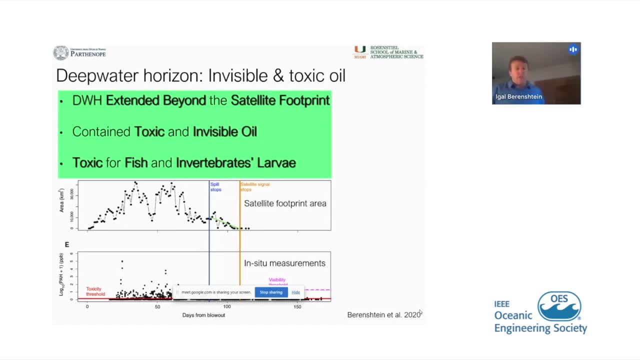 of satellites. the other threshold adopted from a governmental impact report is the oil toxicity threshold, and so these two thresholds allow me to divide the spill into three meaningful portions. can you hide the DD band? did the meet Google banner? so we can see what we? we see some a banner of the meet googlecom. 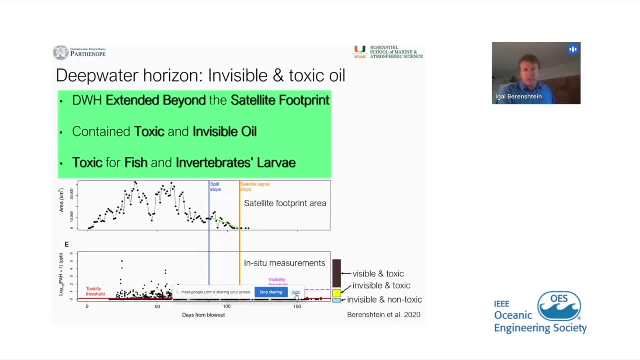 saying that: hi, oh, okay, okay, yeah, yeah, so we can see the second figure. okay, okay, thank you, thank you. can you see it now? yes, thank you very much. okay, okay, thank you. so, um, so this allowed me to to divide the spinning to three meaningful portions: visible and toxic. 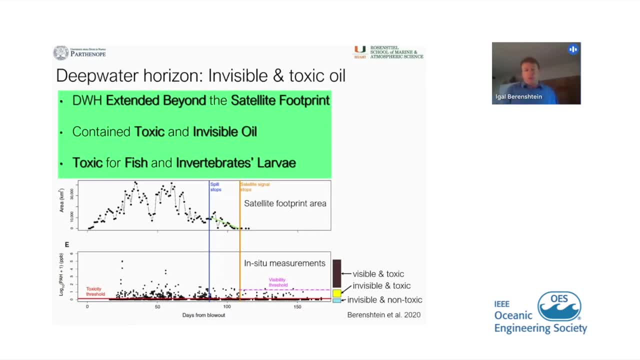 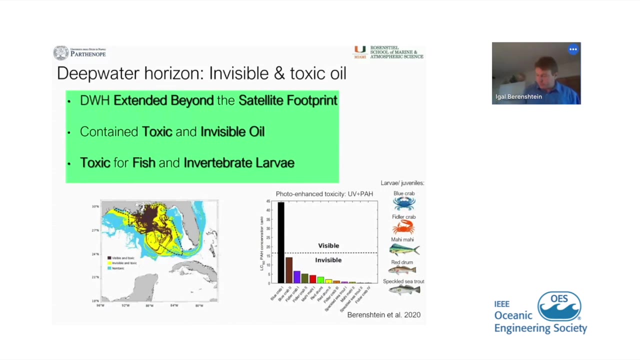 visible and toxic, and invisible and non-toxic. and when we plug in these uh three portions or these two thresholds to the oil spill model, we get a this left map: uh. so the the brown color is visible and toxic, the yellow color is invisible and toxic and the uh the blue color is non-toxic and invisible. 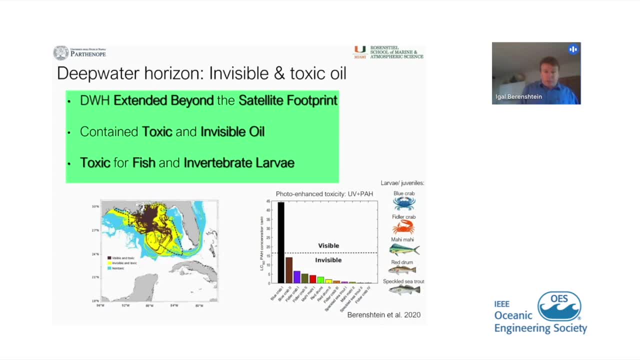 and we can see that toxic uh concentrations, indeed uh extended beyond the satellite footprint and beyond uh the fishery closures. and what's interesting is that what? what uh causes these uh very low toxicity threshold is an effect called photoenhanced toxicity, which is uh toxicity, which is the combined effect of oil toxicity and uv radiation. and if we just consider 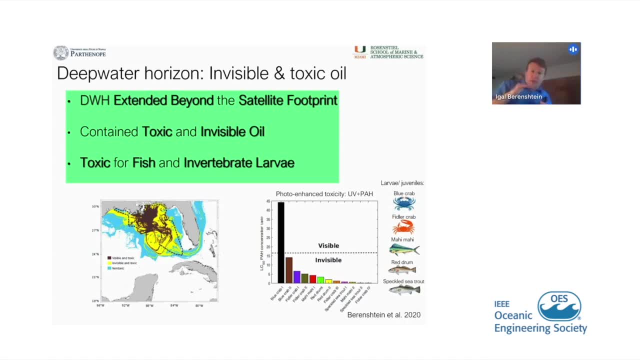 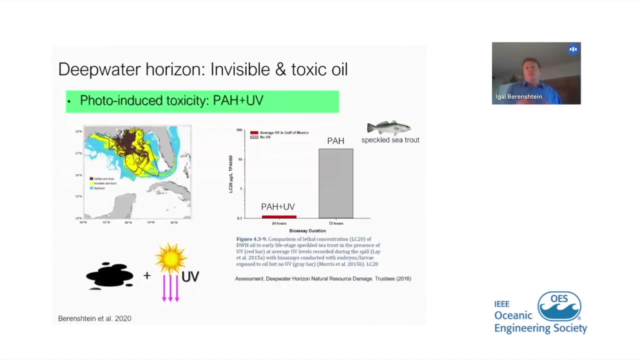 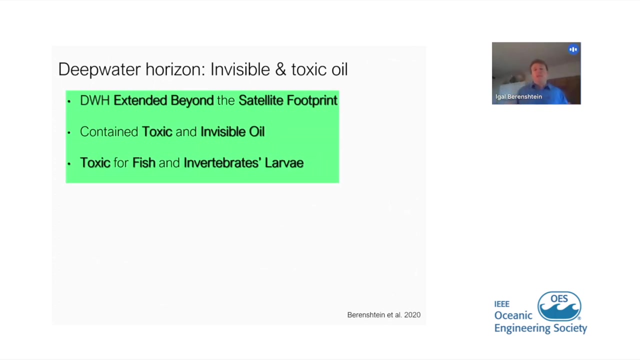 oil toxicity alone, then the toxicity threshold and the visible threshold will be fairly similar and this combined effect of oil toxicity and uv radiation actually can create a hundred times more toxic effect than oil toxicity alone. and these toxic concentrations are especially toxic to early life stages of fish and invertebrates. 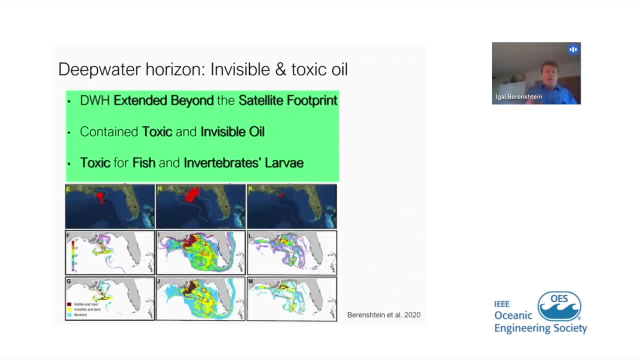 the other thing we can see is that when we uh, when we look at the toxic and visible portion of the spirit, it resembles in shape and in size to the identified oil slicks- cumulative oil slicks- which is uh applicative to to simulate future spills or past spills and to simulate the area. 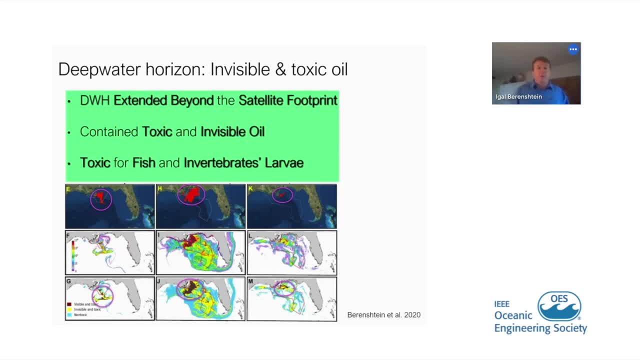 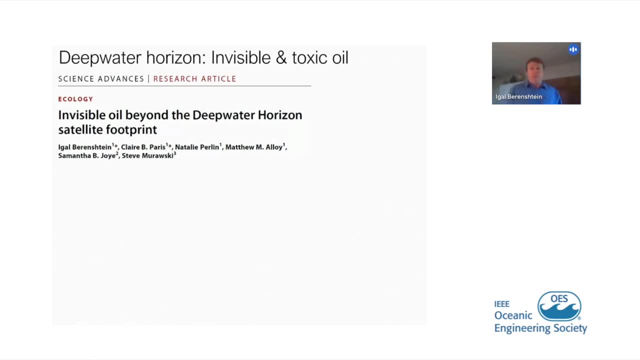 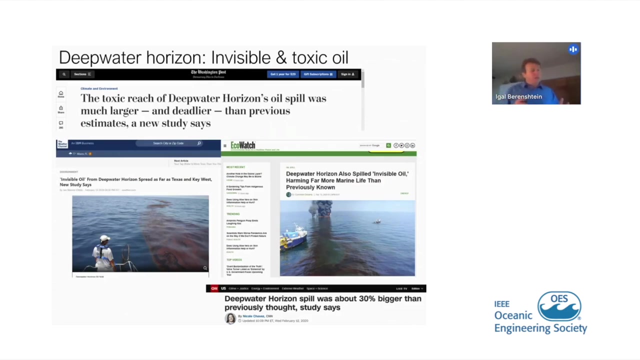 that this the satellite will identify and this was published in science advanced and it really it was covered in many news networks because it really um made us look at the deep water rising in a new kind of approach and but but unfortunately, the effect of oil spillage is not limited only to the 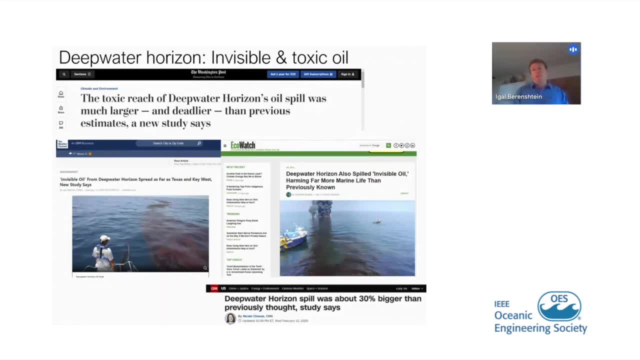 number of animals killed due to the toxic concentration, and it has many more different effects on the ecosystem and on cost of production, and so on and so forth. so it's a very interesting thing when you think about the effects of oil spillage on the fisheries and on coastal populations. 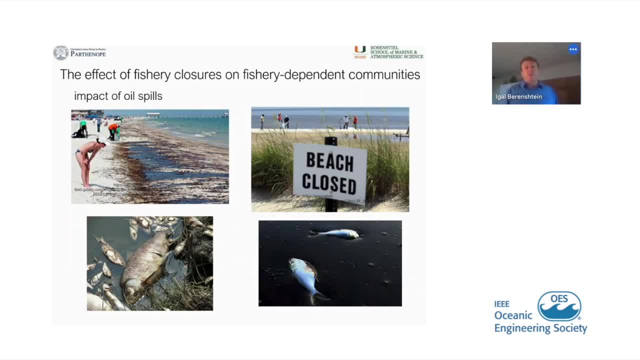 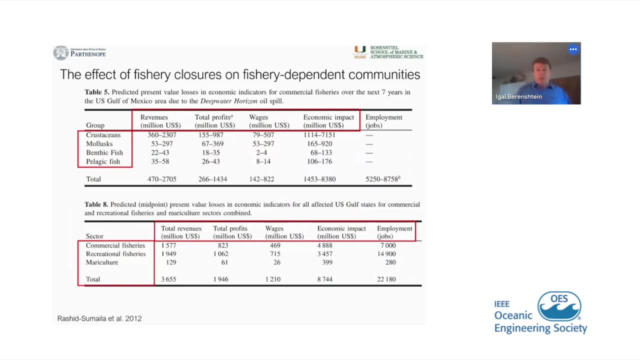 and one of these effects is related to the effect of fishery closures on fishery dependent communities. and what happens is that during the spill, there was a lot of economical damage to fisheries, estimated in billions of dollars, and about 20 percent of that damage is associated to fishery closures, which are the areas closed for fishing due to the risk of 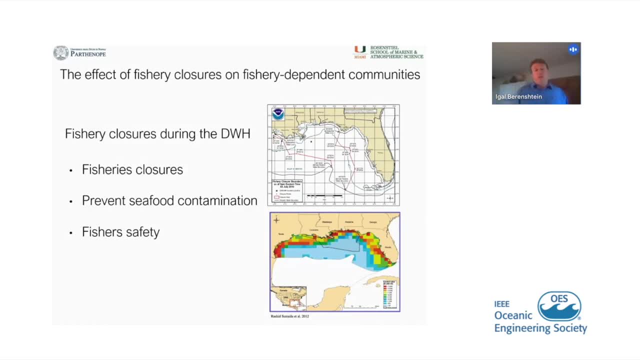 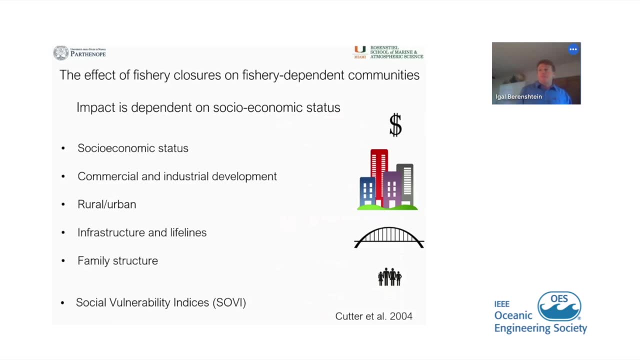 seafood contamination and fishers and looking after fishers safety. but this impact on on a fishery dependent communities differs between the socio-economic status of each community, meaning that if a certain community is such socially vulnerable, then the impact can be more severe compared to a non-vulnerable community which is also not highly dependent on fisheries. so 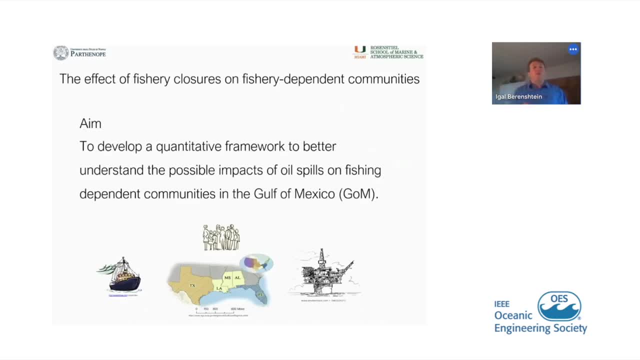 what we did in this study is developing quantitative framework to understand the possible impacts of oil spill on fishery dependent communities in the Gulf of Mexico, and we used three different methods to understand the possible impacts of oil spill on fishery dependent communities in the Gulf of Mexico, and we used three. 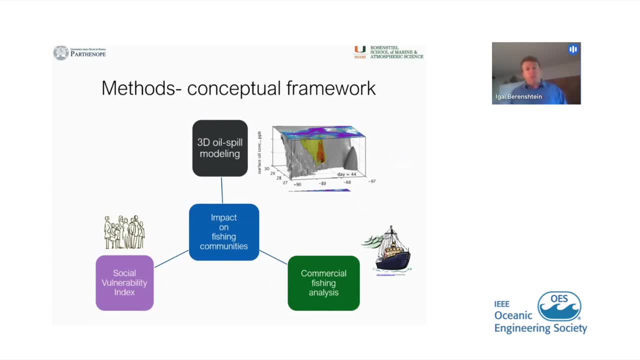 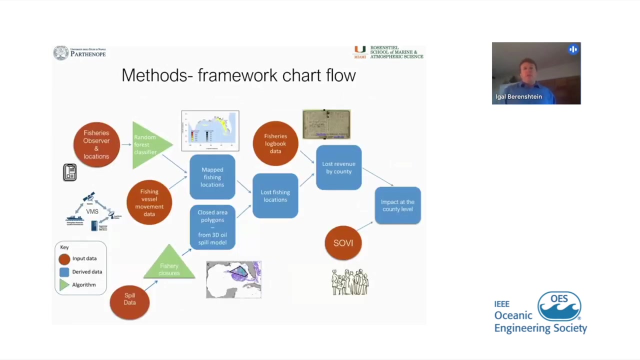 the three main sources of information: the 3D oil spill modeling, commercial fishing data analysis and the social vulnerability index, which looks at various parameters such as family structure, the development state of the community infrastructure, Etc. and, more specifically, what we did? we? we used fisheries Observer data and location. 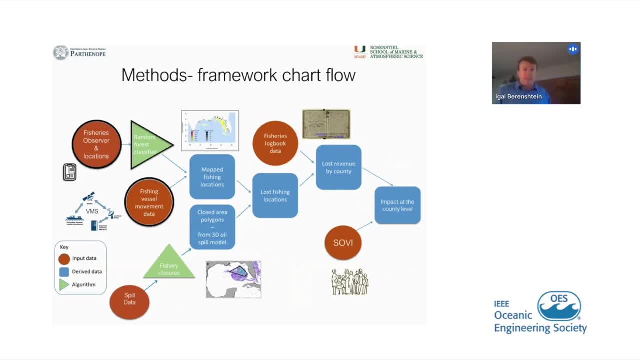 together with fish fishing vessel movement data and we mapped the fishing locations in the Gulf of Mexico. then we use a potential or hypothetical oil spill data and applied automatic Fishery closures based on toxic concentration to produce these polygons that represent we might term the uh cross video on this now. so those are some of the occurrence in in the water. next slide, might you? focus on civil data. so just therefore, I would add that right now we used data for another and then we similar Tapi, to which we don't have been involved with fishамиol. that's gonna come back in detail till next slide. I just want to create more details pictures. I've actually actually flight back to the 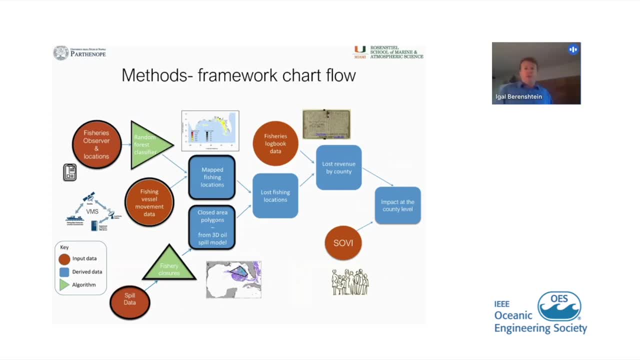 since the potential closures of fishing in case of the spill. From these two sources of information we computed the lost fishing locations and, together with data from fisheries logbooks, we computed the potential lost revenue at the county level. Then, together with the social vulnerability index, 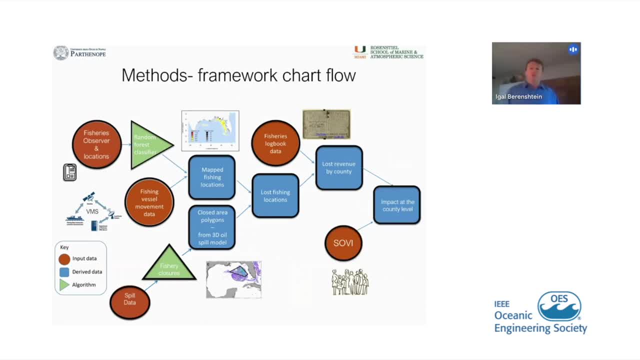 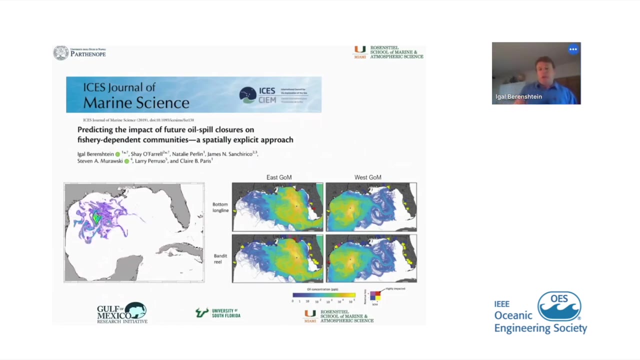 we could compute the impact on the fishery-dependent communities at the county level, considering their social vulnerability state, And this allowed us to map the counties that are going to lose a lot of revenue due to fishery closures, but also considering their social vulnerability. 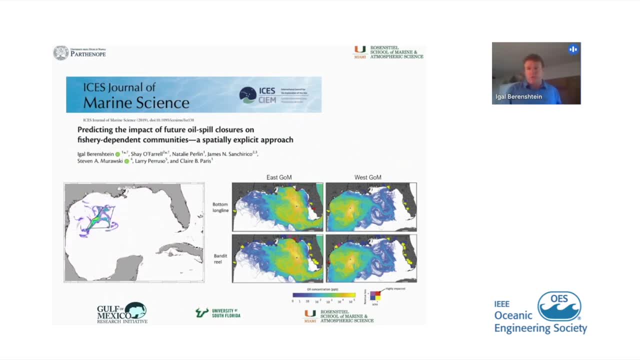 So what you can see in red- the red counties marked here- represents counties that are going to lose a lot of revenue due to the closure, but they're also socially vulnerable And this can be helpful for management and for future planning of oil spill mitigation. 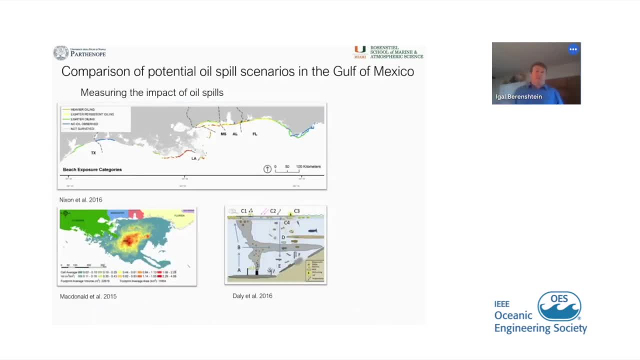 And similarly oil spills such as the Deepwater Horizon. they are complex, They have four-dimensional problems. They occur at the surface, at the water column. There is a deep loom. Some of the oil sinks to the sediment, Some of the oil reaches the shore. 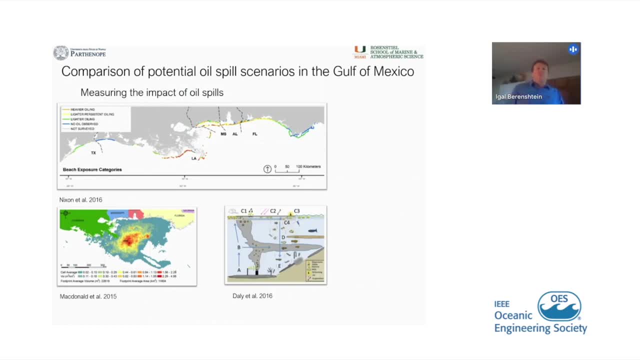 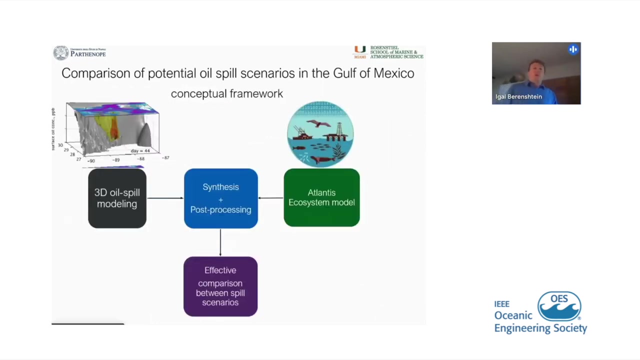 And it's pretty difficult to compare complex spills such as that. So what we did in this project is to compute a quantitative framework for comparing a complex oil spill such as the deepwater horizon. So we use the oil CMS as the oil spill model and transport model. 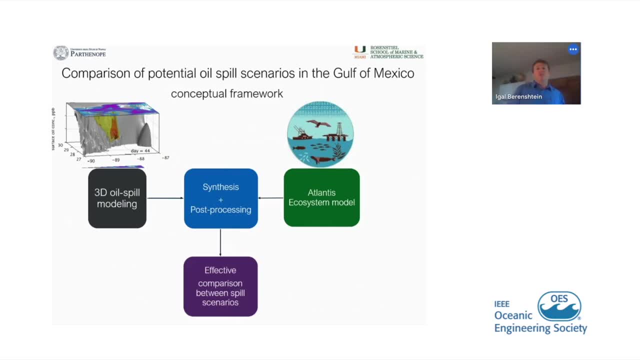 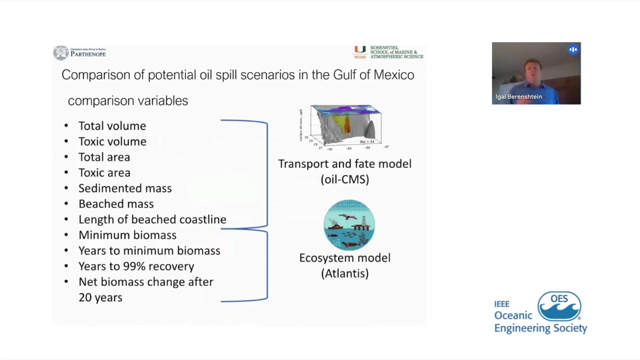 And we use the Atlantis ecosystem model to compute the impact on the marine ecosystem And together, and using synthesis and post-processing, we were able to effectively compare between different scenarios. So specifically, Specifically, the variables that we looked at are the total volume impacted by the spill. 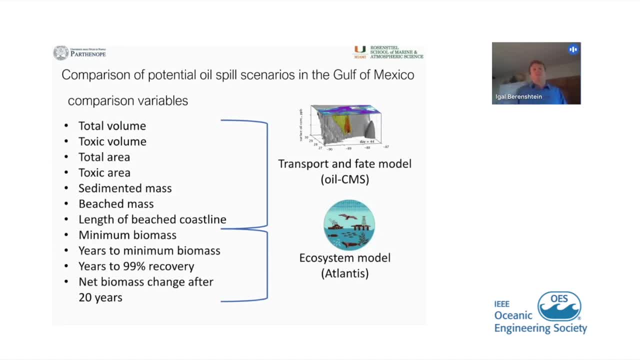 the toxic volume, the volume impacted by toxic concentration, the total area impacted by the spill, the area impacted by toxic concentration, the mass: the oil mass that was sedimented, the oil mass that reached the shore, the length of the impacted coastline, as well as ecosystem. 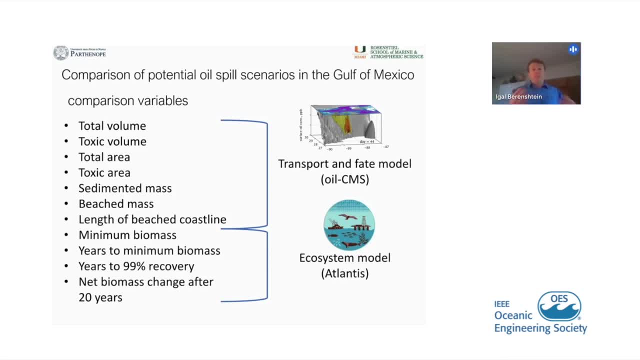 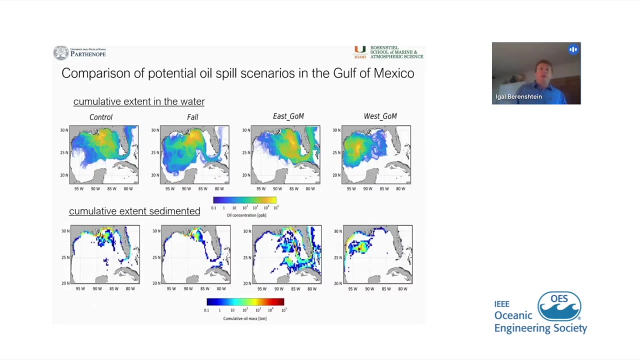 variables such as the minimum biomass due to the spill, the years it took the ecosystem to recover and the net biomass change after 20 years, And we used four scenarios in the Gulf of Mexico, So the control is basically the Deepwater Horizon. 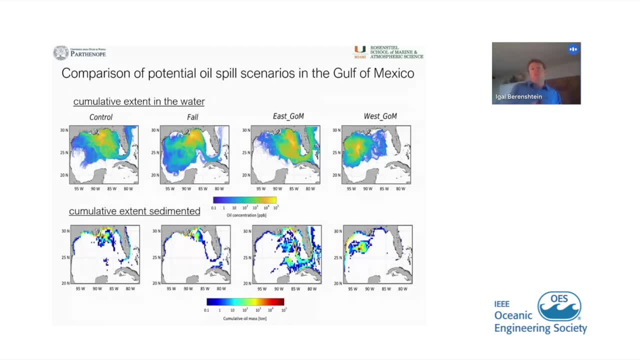 The fall scenario represents the Deepwater Horizon, but occurring during the fall Instead of during the spring. The East Gulf scenario represents a spill occurring in the Eastern Gulf of Mexico, and the West Gulf scenario represents a spill occurring at the Western Gulf of Mexico. 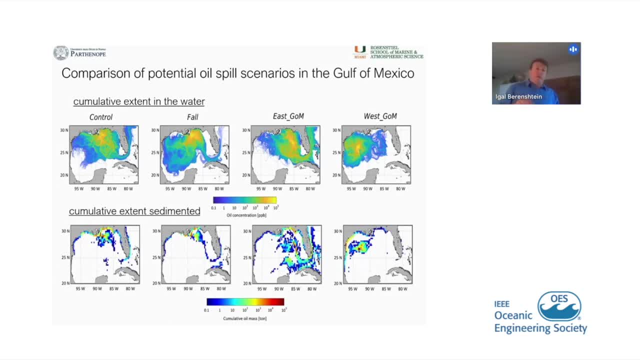 The upper plots represents the cumulative concentrations in the water and the lower plots represents the cumulative sedimented mass- oil mass that sank to the bottom. So what you can see at first glance is that the scenarios are comparable. They are the same order of magnitude, even though there is some variation. 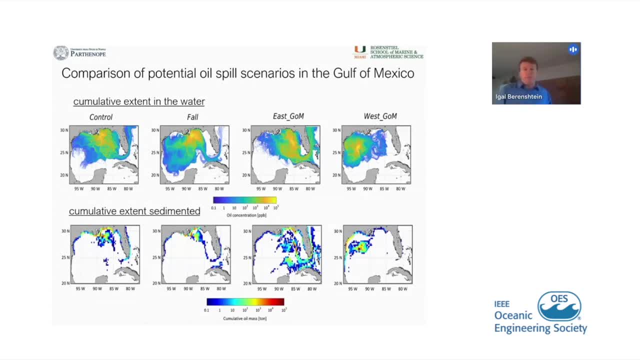 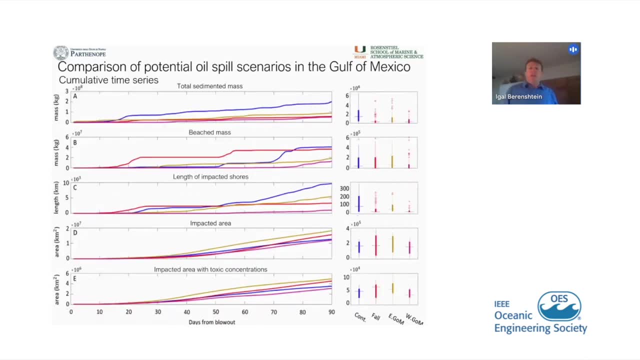 So, both in the sedimented mass and in the water, cumulative concentrations. And if we dive more into the details, we can look at the cumulative time series. And so what we see in blue is the cumulative time series. And so what we see in blue is the cumulative time series. 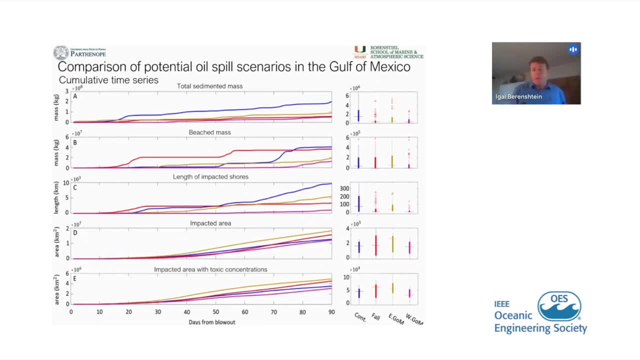 And so what we see in blue is the cumulative time series control, The red is the fall scenario, the brown is the eastern gong scenario and the purple is the western gong scenario, And we can see the dynamics during the simulation. And we can also 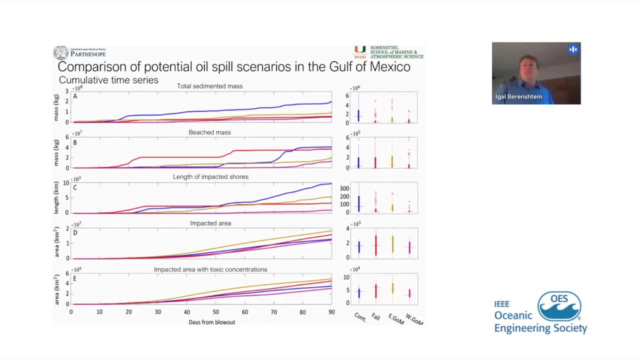 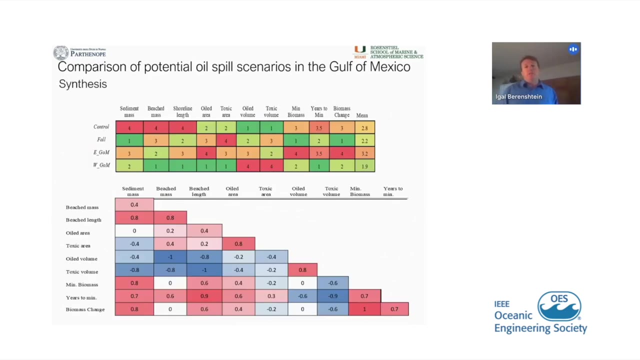 see that there is no single scenario that is either the most impactful or the least impactful. There is variation between the different variables, And then we can summarize this data by ranking the severity of the spill of the scenarios per each variable. So red and high number represents severe, and green and low number, like one, represents. 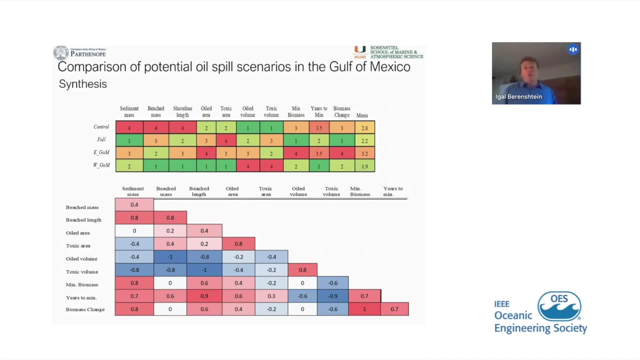 not severe, And what we can see is that the scenarios are comparable And there is no single scenario that is always the most severe or always the least severe, But we can still see that, for example, the eastern gong has the highest score, meaning that a spill scenario occurring. 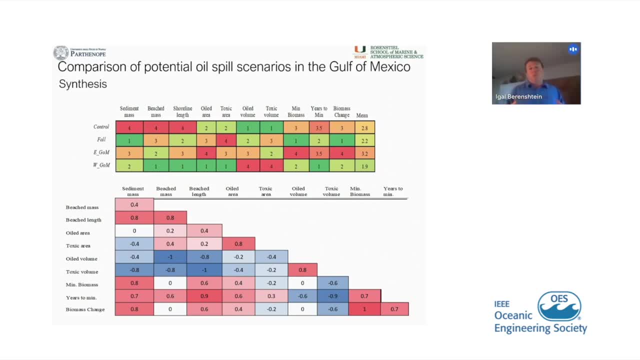 at the eastern Gulf of Mexico will be probably, in total, more impactful than, for example, a spill occurring at the western Gulf of Mexico. And what we can also do is look at the correlation between the different variables, or the tradeoff. So it makes sense, for example, that there is a correlation between the sedimented beached. 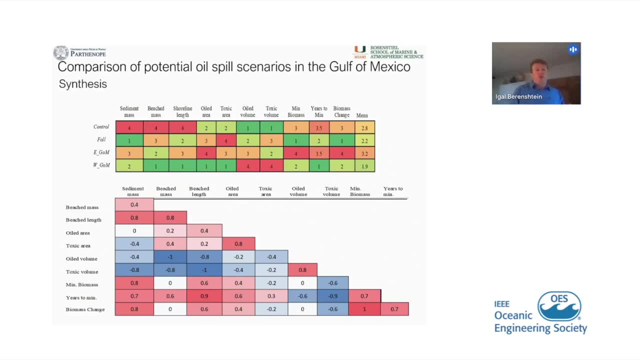 mass and the shoreline length that was impacted by the oil spill. So the number here is the correlation coefficient between the different variables, Okay, and for example, there is a negative correlation between beach mass and oil volume, and that makes sense, because oil that reached the shore is will not be in the water column and therefore the 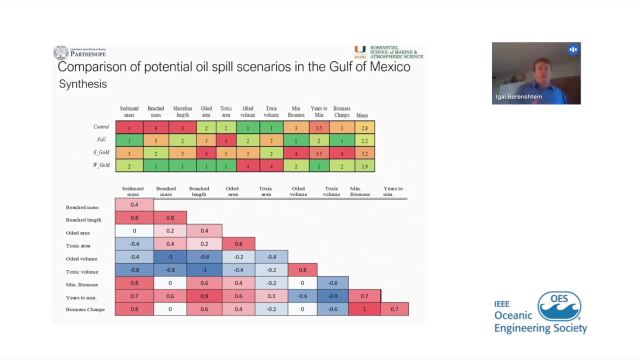 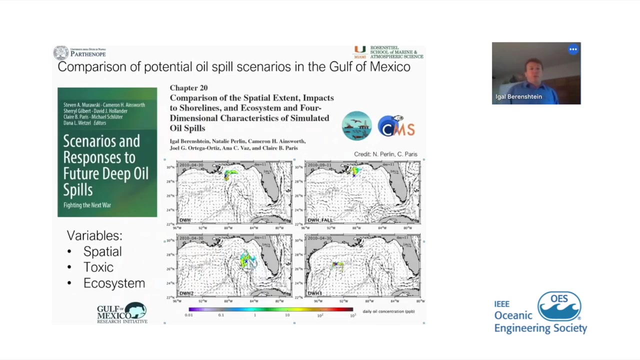 volume of the water that will be impacted by the oil will be smaller, and so this allows us to kind of have a general view at the dynamics and provide some meaningful insight within this complex problem, and this was published as a chapter in the book scenarios and in response to future deep oil spills. 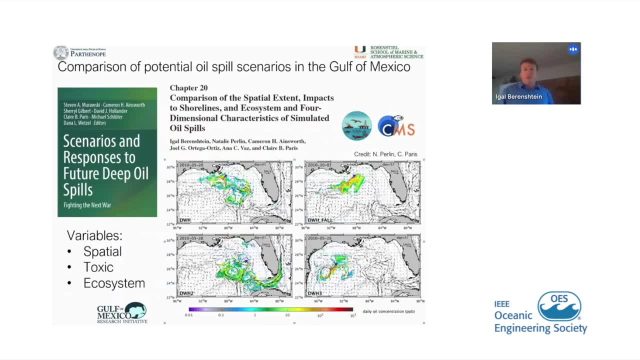 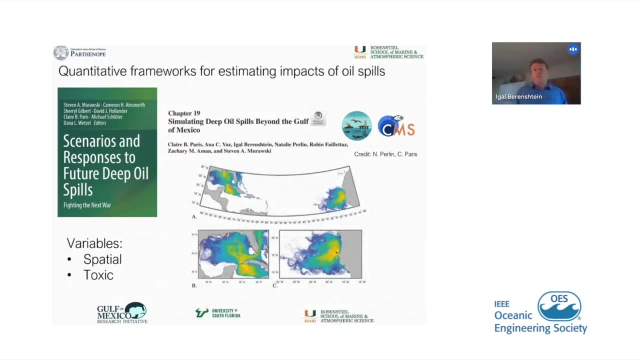 and we used a similar approach to to look at possible oil spill beyond the gulf of mexico, one in cuba and one in west africa, in senegal- and we can see the size and the effect of these possible oil spills, which is immense, and that was also published. 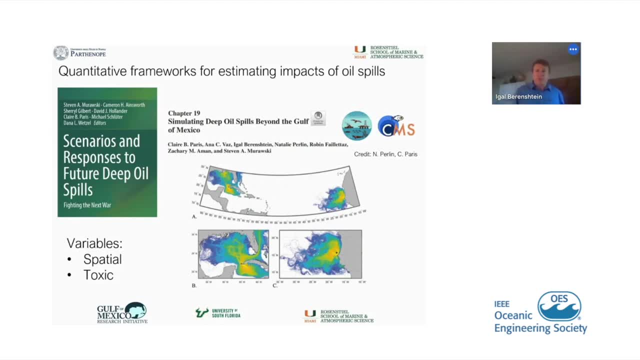 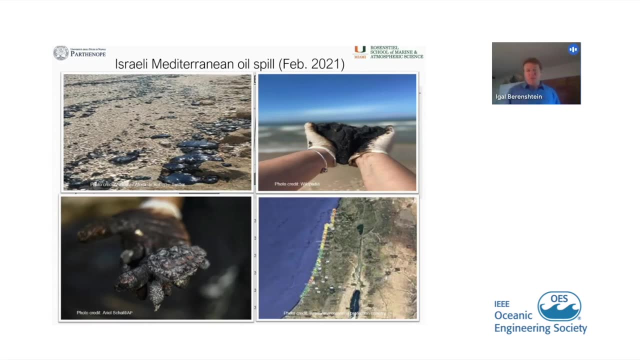 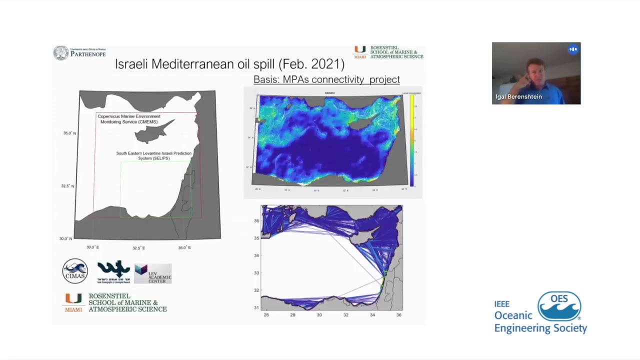 in in that book as a separate chapter. um, and i will talk a little bit about the spill that we had a year ago. um in israel, and what allowed us to reconstruct this spill is is a different project in which we compute connectivity level, connectivity between proposed marine protected areas. 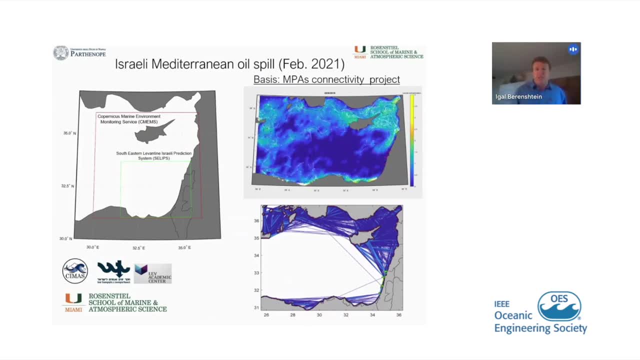 in the eastern rope, in the eastern mediterranean, and so we had the oceanographic data for that region. and then when that spill happened, uh, it was fairly easy for us to to reconstruct the spill, and we collaborated with with researchers from erikman university, tel aviv university, the israeli meteorological service, to compute the spill. so we 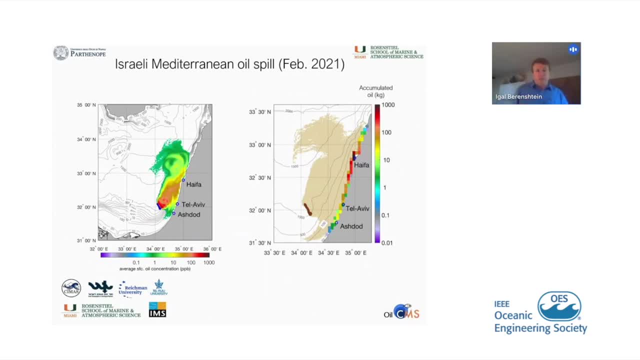 identified the the oil slick location during a february 11 last year and from that oil slick location we uh modeled forward in time the spill dynamics and again computed the oil concentration in time and space, both in the water and what was sank to the sediment and what reached the shore, and that 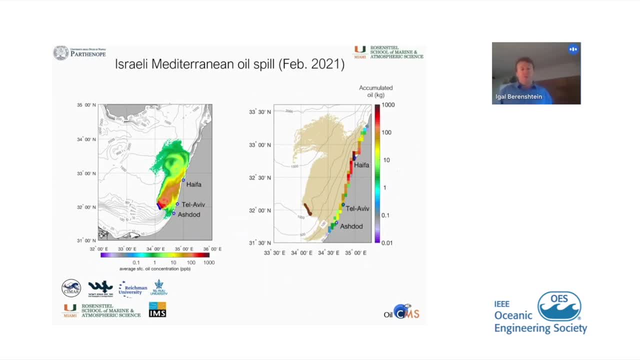 fitted well with what was observed, observed in the field. so during that spill last year, the entire coast of israel and some of the lebanon coast were contaminated by tar and by oil, and this this reconstruct the spill and what we are. we have recently completed a manuscript, that that calculates the economical impact of that spill and 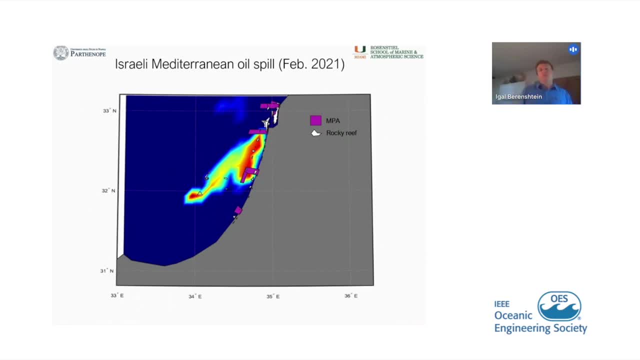 i will be working on a manuscript that computes the ecological impact of that spill, so what you can see is that this spill overlaps with marine protected areas and with rocky reefs, areas which uh harbors more biodiversity, and this, together with larval abundance and connectivity, have to be considered when we talk about the impact of that spill. 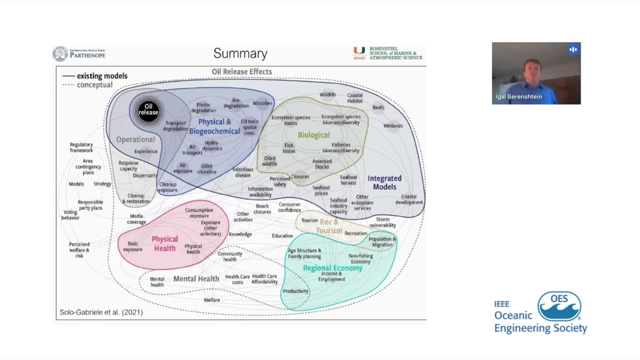 and so, to summarize, um, the scientific world realized that oil spills are complex events that are not only limited to the oil transport itself, but they contain physical, by biogeochemical components, biological components, economical components and physical health components. and and what we did in the, the projects i presented here, is to to 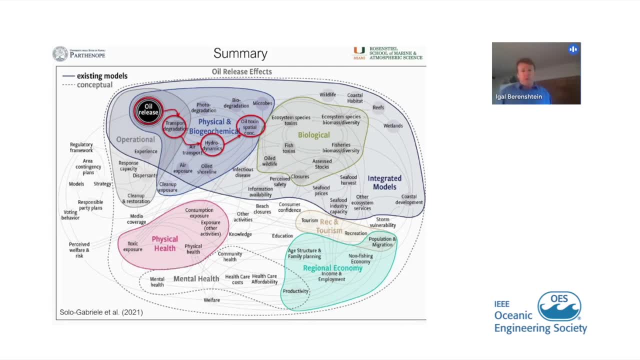 quantitatively connect different aspects of these separate components related to the physical and biological, any chemical components and the meaning of the sauce in and u component, as well as the toxicity and the impact on fisheries and impact of the closures on seafood harvest and on the income and employment of fishery-dependent communities. 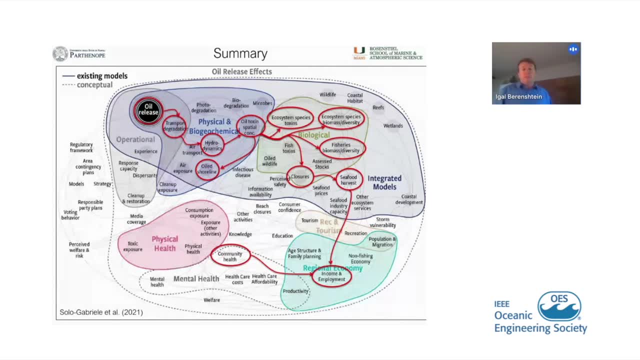 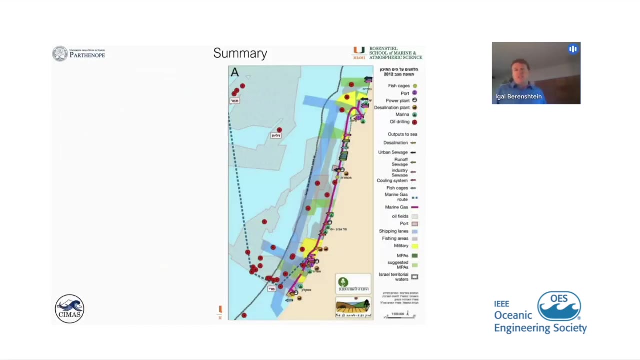 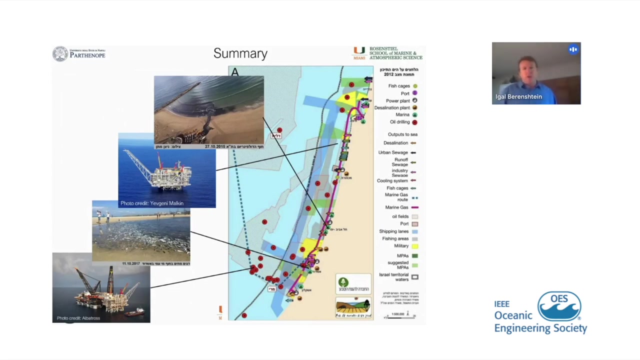 And this is an important step into a better and holistic understanding of such complex events such as the deepwater oil spill, And in the Eastern Mediterranean we have a very crowded sea with a lot of anthropogenic impacts, including oil and gas rigs, as well as terrestrial runoff. 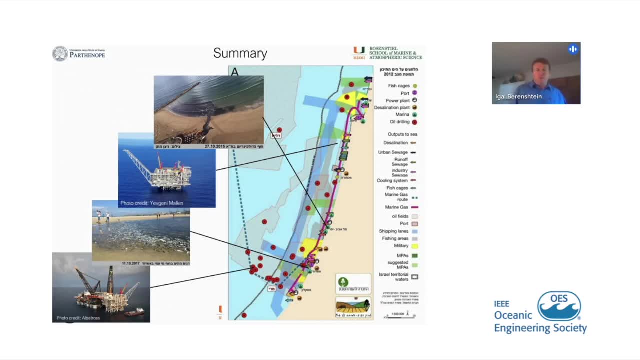 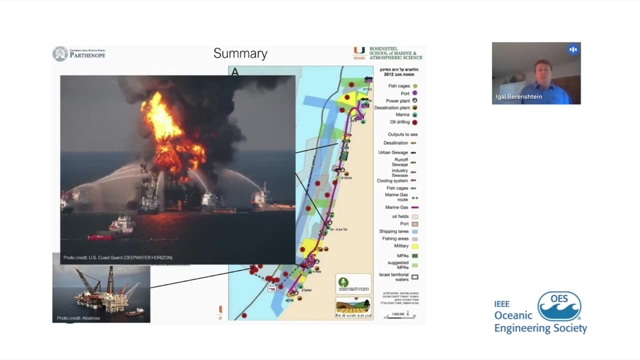 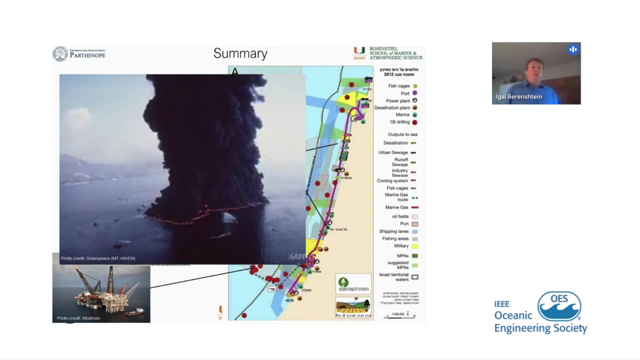 And the spill is not only the pollution is not only limited to that spill that I presented. These are chronic, Okay Okay Pollution that we need to consider and, of course, an event such as the Deepwater Horizon or an event such as the Empty Haven that occurred in Italy in 1991 can reoccur and contaminate. 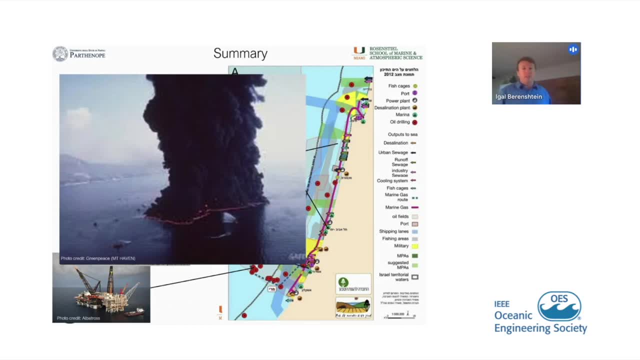 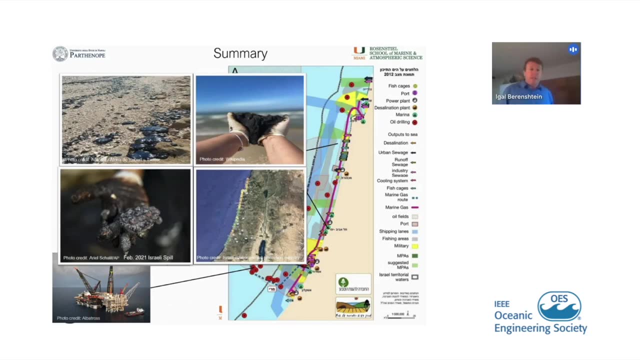 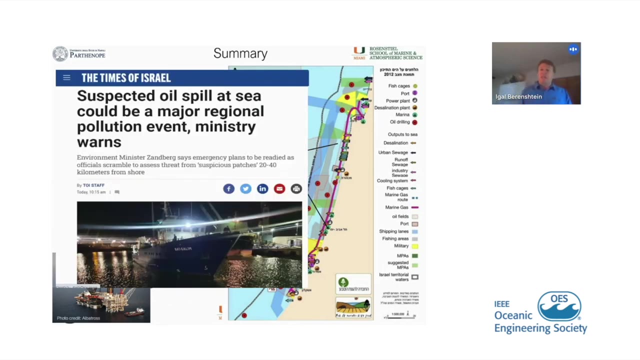 entire regions in the Mediterranean And, of course, the event occurred last year is a good reminder and a good lesson for us to be prepared for such event. And actually, only yesterday there was an identification of an oil slick in front of Israel and we're still not sure if it's going to, if it is indeed oil and if it's going. 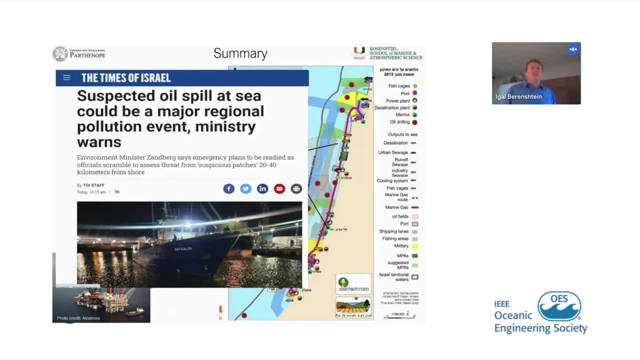 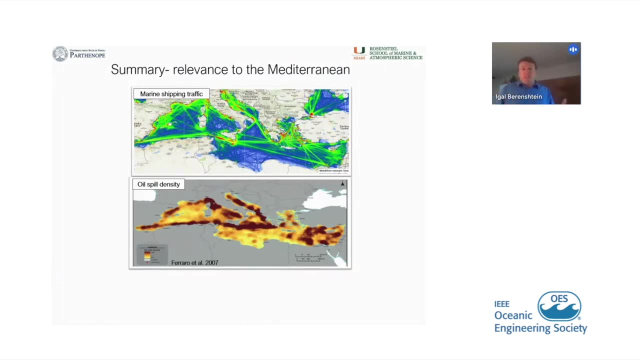 to contaminate the shore, And so this is events that are frequent and abundant, and we need to be able to account for them, both environmentally and economically. So, if we look at the Mediterranean as a whole, it accounts for, although it accounts for. 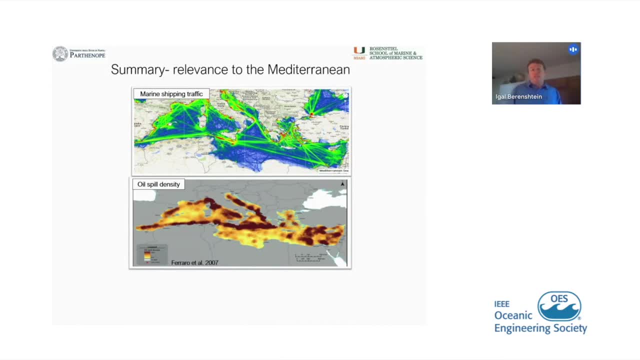 less than 1% of the ocean area. it encompasses 15% of marine shipping traffic. It is very dense in marine shipping traffic And with the traffic there is, of course, oil spill events which are very abundant across the especially the Northern Mediterranean. 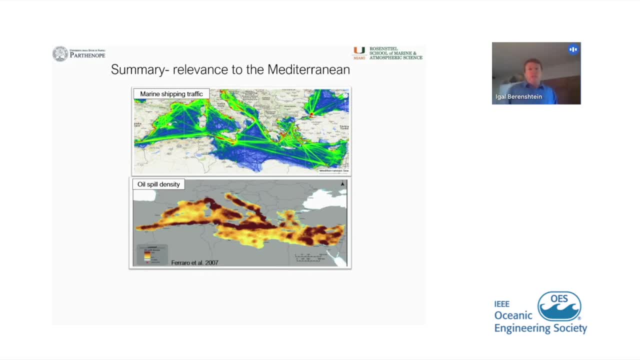 And the Eastern Mediterranean, and we need to be able to account for this pollution. So if we're, if we want to study the Mediterranean ecosystem, we cannot ignore this chronic and severe pollution. We have to take that into consideration And, hopefully, what we need to do as scientists is to collaborate with, you know, with the 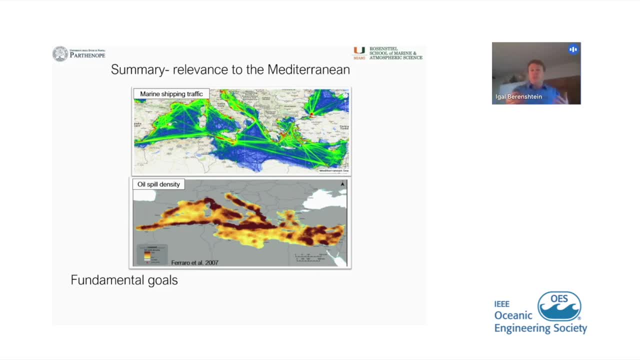 Mediterranean. So engineers like you, with marine ecologists and marine ecosystem science, to form collaborative frameworks to be able to answer two fundamental goals: One is to quantify the effect of marine pollution on the marine environment And the second is to quantify the effect of marine pollution on coastal human population. 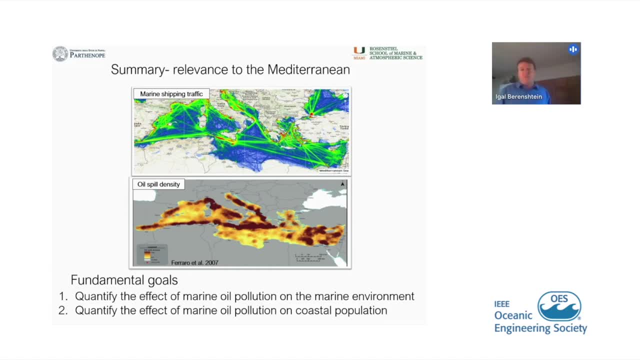 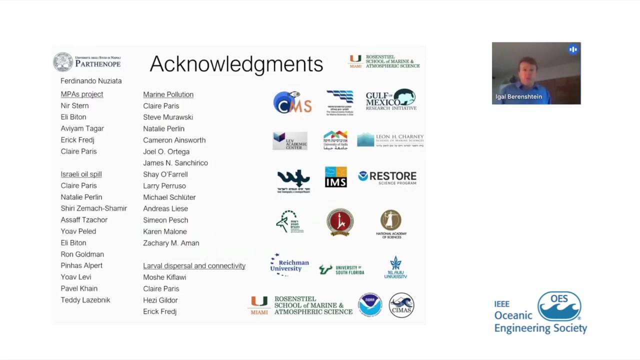 And this is critically important given the tropogenic development, the increase in oil related activities and the high toxicity of a high impact and high toxicity of oil pollution, which is currently not accounted for properly. With this, I would like to thank you for listening. 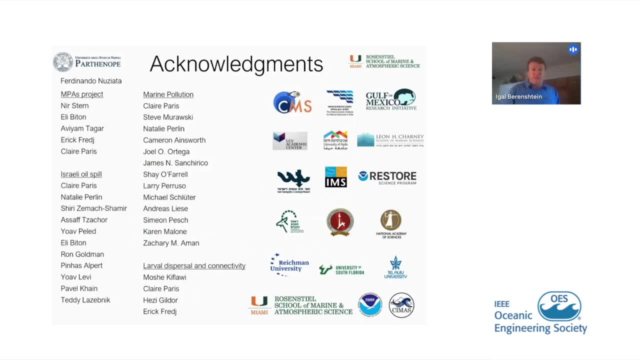 I would like to thank you for inviting me. Thank you, Thank you, Thank you for giving this talk, And I would like to acknowledge all the collaborators in the different projects and the funding agencies, And especially Claire Paris, Steve and Natalie Perlene, who were instrumental in leading. 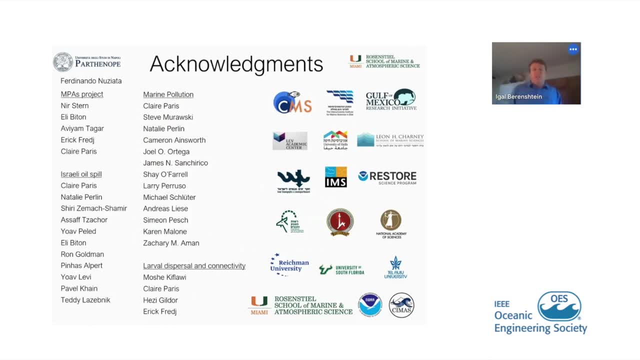 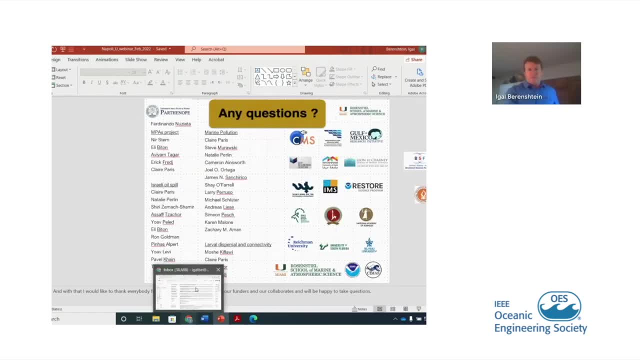 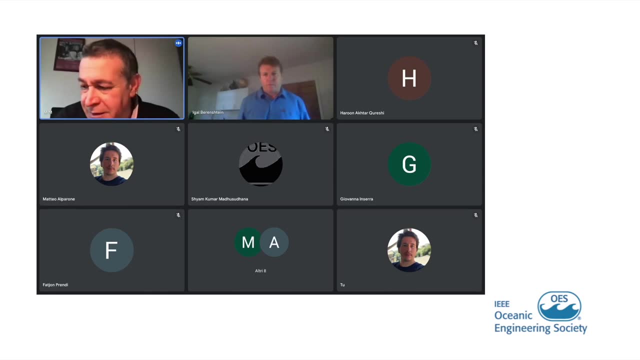 i have a first question, but i i invite all, the, all the audience to to to my question. of course, when you compare the, the, the, the analysis- let me say satellite based and and on ground, you didn't- of course it was, it was obvious- give too much details about the both techniques. 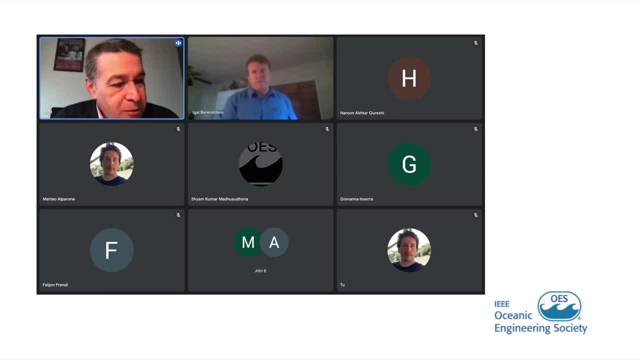 and it would be, uh, would be nice to, to learn something very, very general at least about the remote sensing activity or idea monitoring one and, of course, the in-situ one, because, of course, when you say the label, for example, i remember the, the, the one of the graph, key graph that i 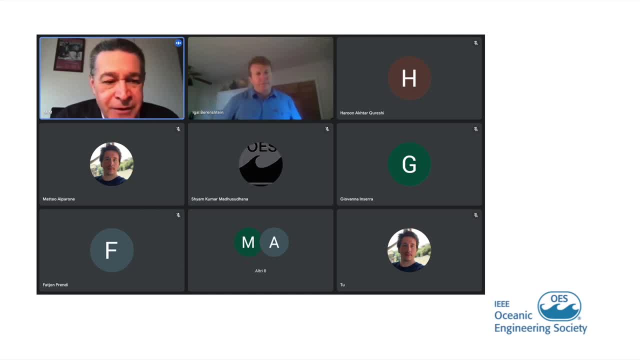 asked you to show the lower part. of course, this comparison is always dependent on the technique you use because, of course, the sensitivity of the different techniques or procedure or instruments at the end- yes, that's, i just want to comment. i mean, give some more, i don't want to take all your. 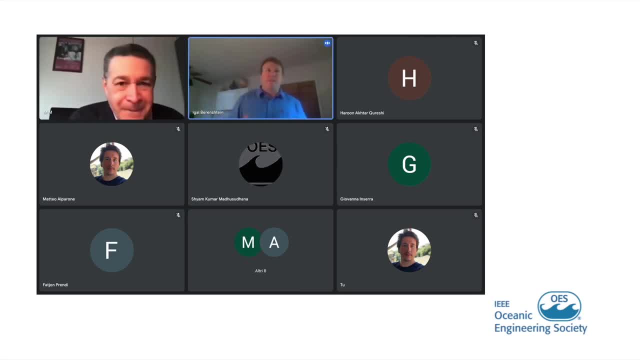 time. but no, no, that's fine, that's a good question. so so basically, the the, what i call the remote sensing is not only remote sensing is mainly the sar satellites, but it's also um airplanes that flew above the area and identified visually snakes and a visual identification from both, so they. 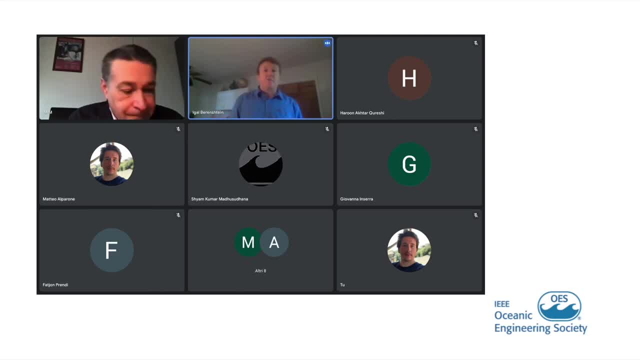 combined these, these sources of information, and they created what they call nest, this anomaly polygons. so they have like daily polygons where uh oil was detected in either of these techniques, but even in the israel case, also in the institute. okay, so you know, in the israeli case it it was. 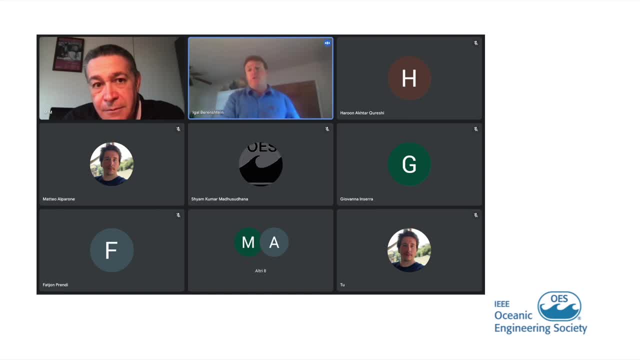 only the, the sar identification for that day. there were different days, so a few days before the there's, there's a different techniques. i think it's just like the um multi-spectral imagery, but for that specific date, uh, i think the, the, the multi-spectral imagery, was not available and, uh, they use sar and i. 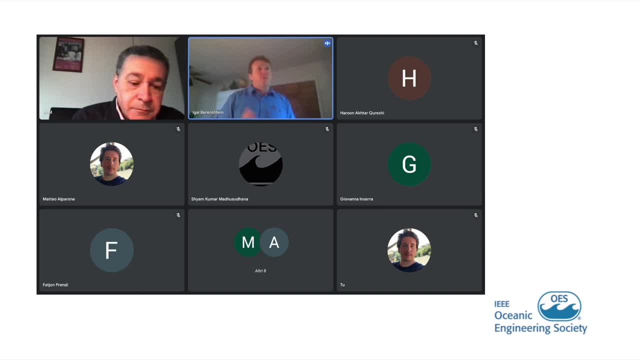 actually also, uh, um, you know, use the satellite data to find that slick and and validate that this is indeed the shape and the, the, the size of of that slick for that day. um, so it's uh, you know, it's uh, uh, from copernicus, it's the sentinel a1. 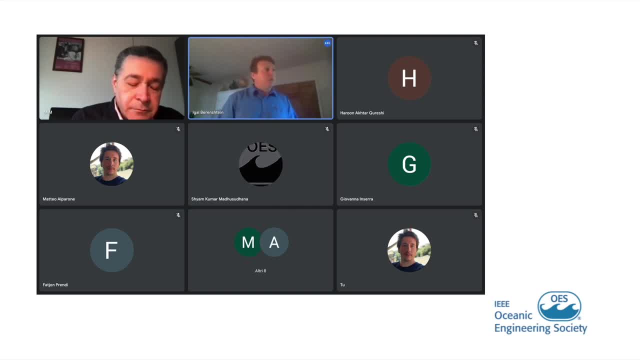 a sar, a vv polarization. i think it's what's normally used for for a oil slick detection. so single pole, single pole analysis, yes, okay. what about the ons on site? so on site in the uh. so we, we didn't have anything for the mediterranean spill, there wasn't any. 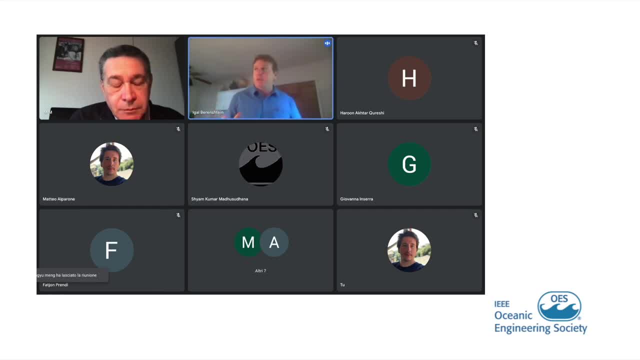 measurements. but for what i presented for the gulf of mexico, there were um in-situ samples. so they, you know, they, they uh, the employed the niskin bottles, they took water samples and they sent it to uh to the lab to do gas uh chromatography and mass spectrometry to measure the total petroleum hydrocarbon. 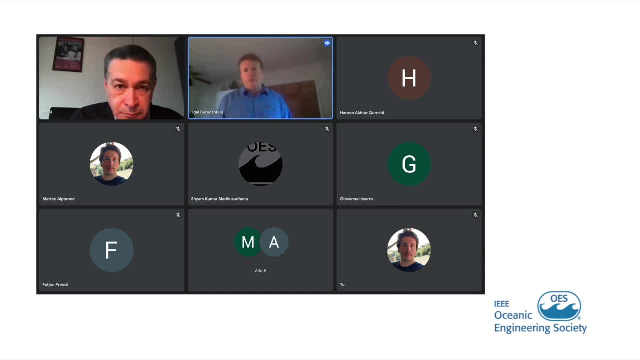 concentration and the polycyclic aromatic hydrocarbon concentration. so there's like a huge database. there were like probably tens of ships that took part in this immense uh sampling something. let me say, yeah, it's a real sampling. you're saying, yes, it's sample, it's real sampling, it's not remote sensing, it's real sampling. and yeah, and i think, 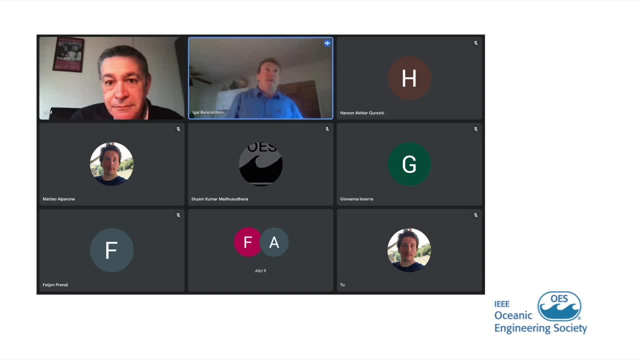 and that's for the what we call the gulf science data. that was, these 40 000 um water and sediment samples and these independent studies. so each used a slightly different technique. some used measurements. there were like various techniques, but the bottom line is that these techniques indicated the 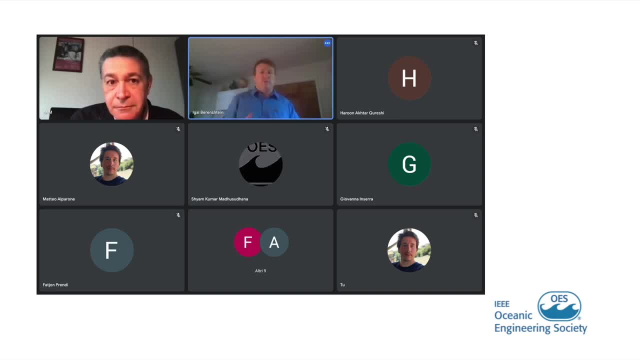 presence of oil at these locations. so so i i mark them as as crosses. but they use different techniques and and some somewhere um at the beach and somewhere at the sediment, somewhere at the water column, some did their um fingerprinting, so they identified the, the exact structure of the macondo oil to to make sure that this is indeed oil from the deeper horizon. 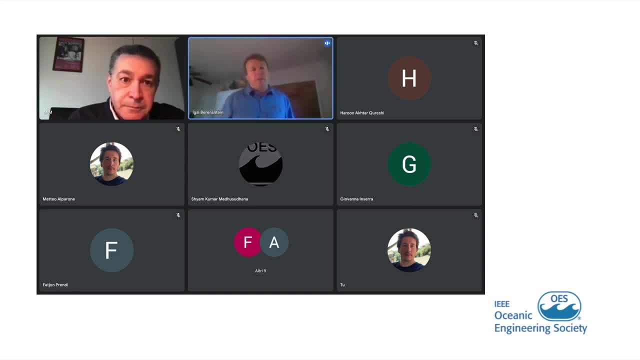 so there's a variability in these, uh, independent studies. okay, i understand any other question comments. hey, like a question, are you there, andre, andre hi, nikal nice to meet you? very, very interesting presentation, thank you. just a curiosity about the: the recent oil spillage that happened in the. 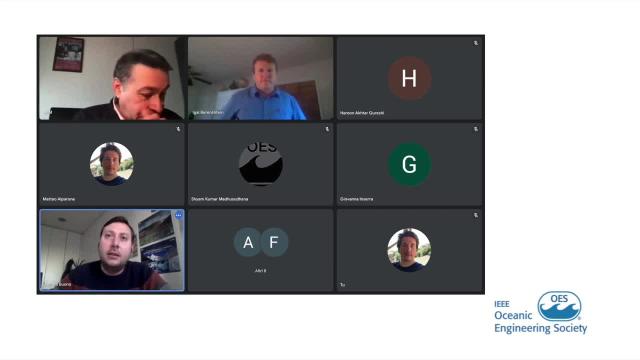 there were an underlying another water pipeline that release a lot of oil over there. so yes, i'm updated information. i know it's far away from the group for mexico, but no, i i actually didn't look too much on that spill. i i was, you know, i was kind of, uh, i looked at some spills that occurred. 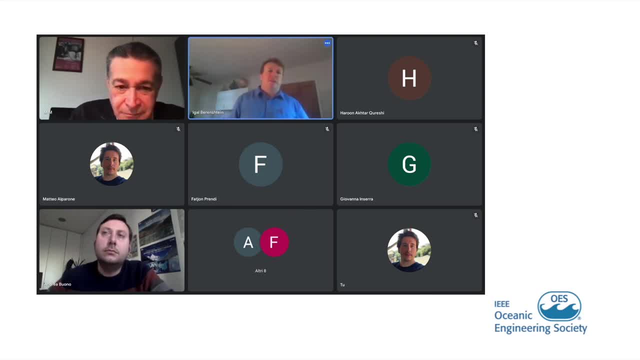 in the past years, but not specifically on that spill. but uh, i don't know. do you have like a specific question? no, i, since the the the phenomenology of the oil spill very similar to the deep water horizon, since it was a broken underwater pipeline. so it was interesting to. 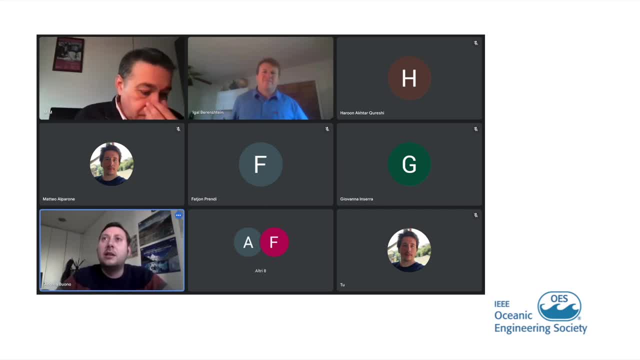 compare after almost 12 years if some advancement in use of both ground remediation activities and the support of satellite measurement, it was improving in the last decade. yeah, um, so i i don't have too much information about that. do you know what the depth of that spill? um, i read something, but there are from the the news online journals, but 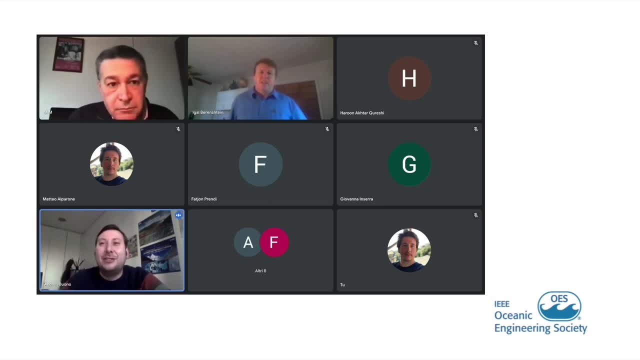 they say very different numbers, so i think it's not an official source of information up to now. so, so so there's a big difference in in like ultra deep spills and and ones that are, uh, occurring fairly shallow. so, for example, there was the ickstock spill that occurred in 1979. 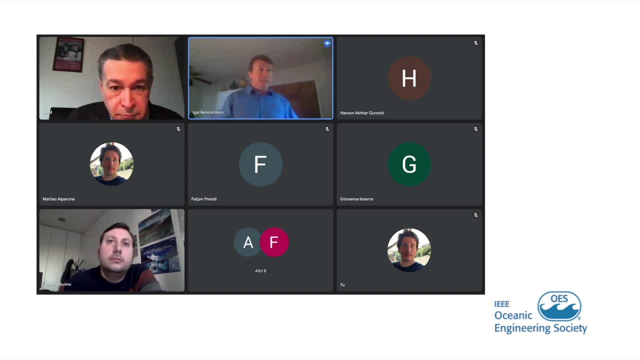 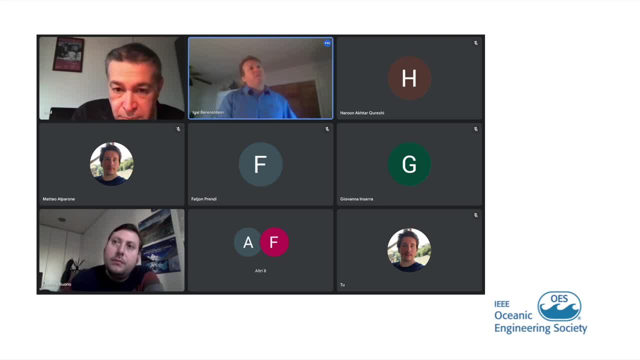 of the majority of the oil, just um went up to the surface and then uh transported to the, to the area of of texas and, and you know, the rest of the us gulf states, and so that is a fundamentally different spill than the deep water horizon which uh was like at the depth of uh you know. 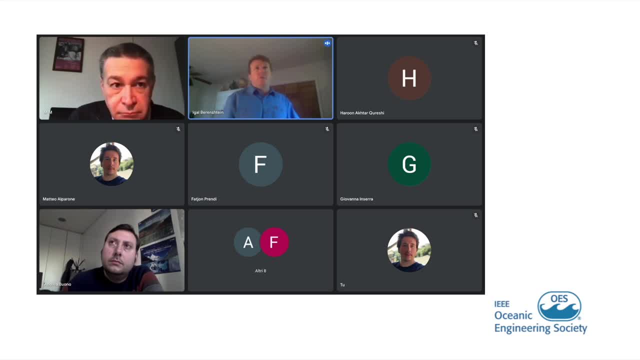 uh, remember correctly it was 1500 or something like that, very deep uh and so for. for that, these conditions, because they're like a very high pressure underwater, then much of the oil is is captured in depth, so there was like a deep room in in 1200 meters. that, uh, that was very wide and 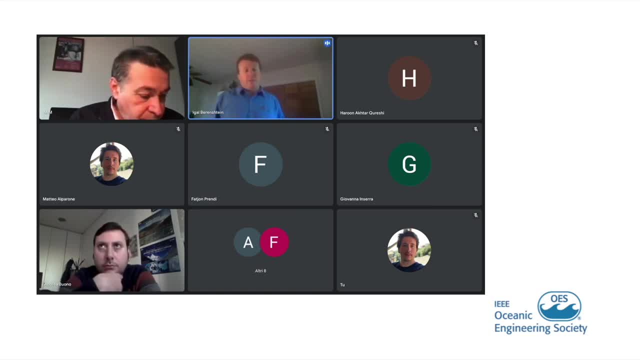 very long and- and that was something that discovered- uh, was discovered during the deep water horizon and it is very unique. it will not occur in a in a shallow spill. so that is kind of the that's why i asked for the depth of the spill. so there's a lot. 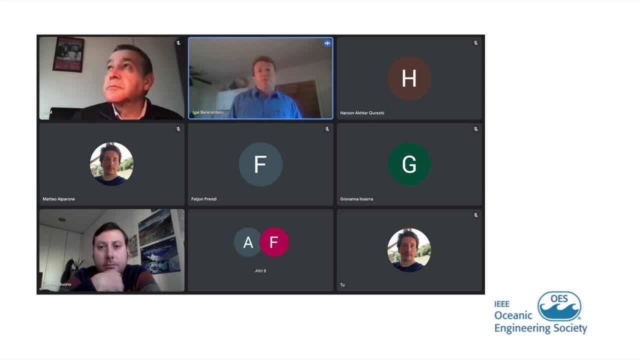 of difference if the spill is very, very deep. okay, thank you, reagan. thank you even for the temperature, you know. yes, yes, of course this is a challenging task. anyway, whatever is the remote activity, which is the sampling activity, or i understand what you say- if you operate, not in. 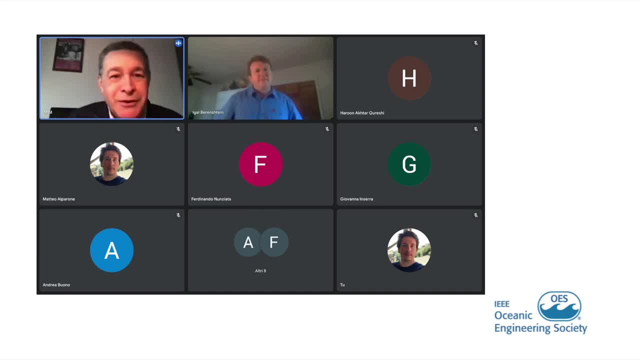 scientific terms, even in some way supporting the operational activity. you try to do your best and of course at the end the scientists are involved, even to make a paper, but in that moment you try to do your best, whatever it is. so it's not a coordinated experiment that you design. 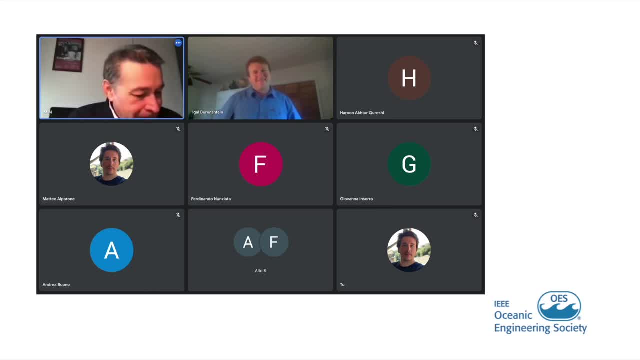 on purpose. okay, let's make- let's put this clearly- uh, but my point is to to of course, you have three ingredients. let me say basic remote sensing is helpful, but of course, as you know, we are much more uh in favor of polarimetric uh measurements. 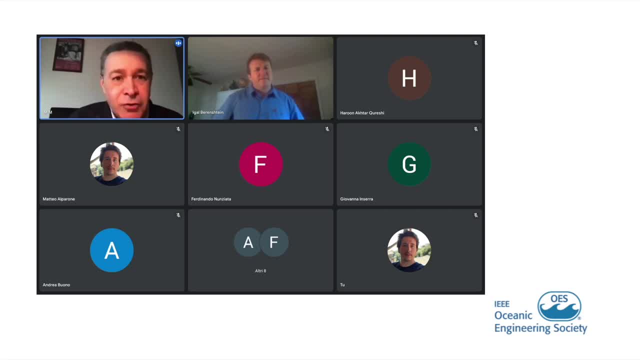 sour measurements, although i understand some cases it's not easy to have them in a high quality and enough high density in temporal and spatial density. then you have some measurements on site, whatever it is, uh, some health and safety measurements, and sometimes you have biometric measurements and then you 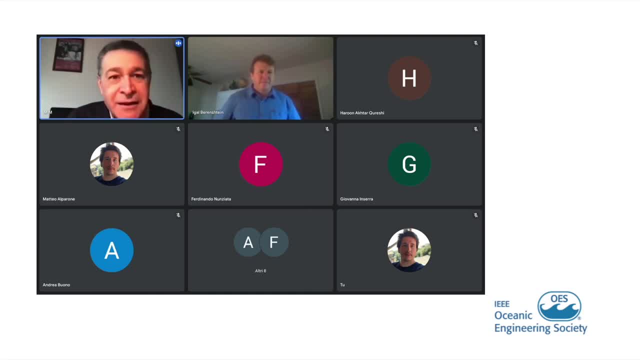 use a large scale sensor camera and you can actually work with multiple lenses. to, you know, take the samples and work with multiple lenses. i would say that this is a kind of a sort of a fat каких, more physical type of thing or, um, you know, a very, very difficult task of sampling uh, uh, ufb instruments. 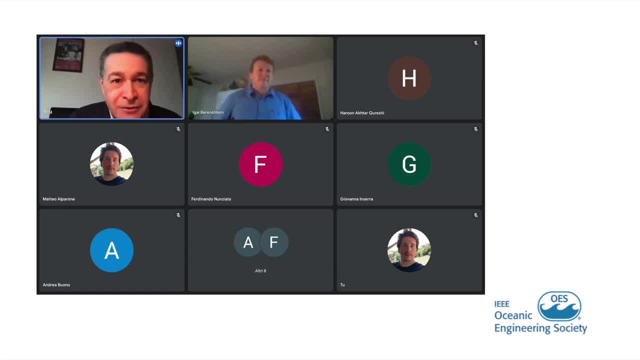 which is critical, but of course this must be coordinated, at least theoretically, taking monitoring the most critical areas. think about the gulf of mexico. this was kind of a gigantic oil spill. you you may even benefit of some transportation model. You mentioned this. I don't want to say that on the scientific side. 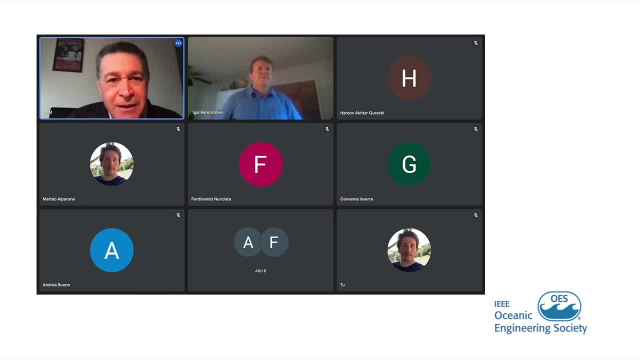 it is. on scientific side, anything has pros and cons. But my point is simple: In a real task- okay, you know I don't want to say operational, but helping the operational guys- how much was your feeling that? let me say the people on the ground- 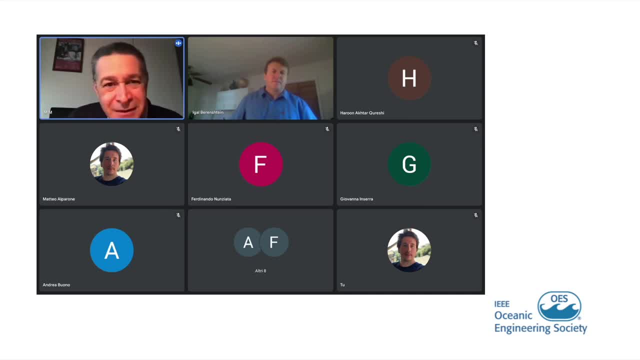 the real operational trusted you or the scientists or the remote sensing guys. because that I want to share my feeling with you. But let me say you understand your advice. I don't want to say they are not perfect, they are real. 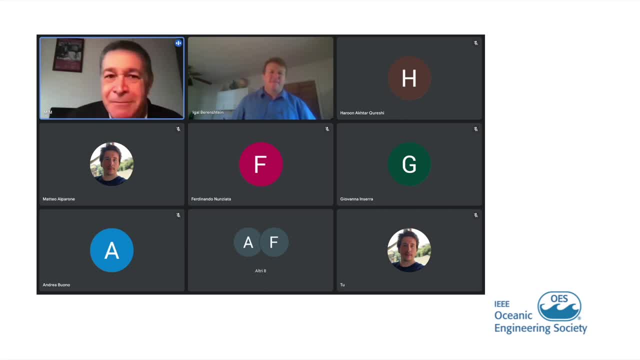 but coming from the model, coming from the sampling, coming from, let me say, some remote sensing analysis, that analysis which is the real benefit that the people in charge of the operational services trust you- not you personally, of course, I mean. yeah. 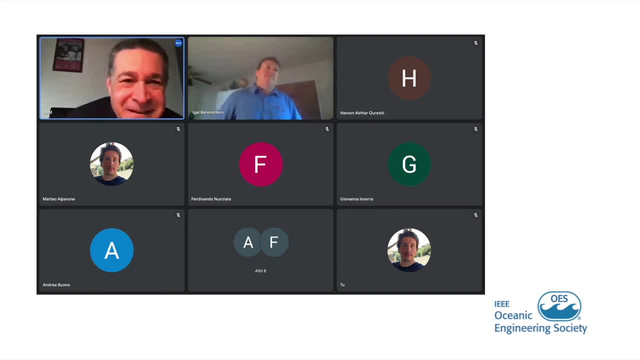 It's the science. It's the science theme, let me say science theme. It may be good, but do you understand what I mean? Yeah, Yeah, Well, we have to take into account the fact that you know I came on board seven years after the spill and you know. 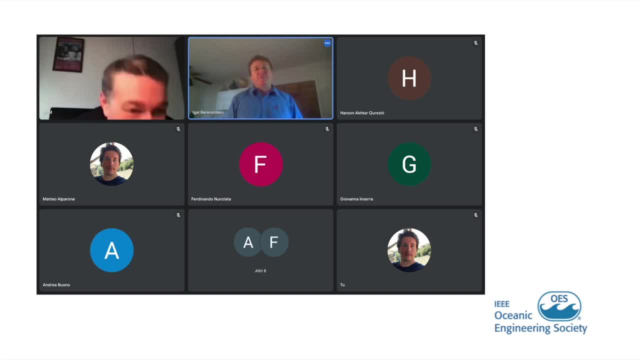 the operational part was over a long time ago, But Israel was not Oh well with Israel, because I didn't. I didn't take part directly, I was not there as well, but they did. you know, there was some kind of information transfer. 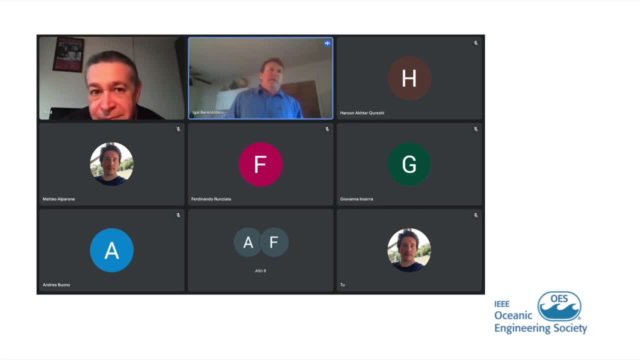 But I think the point is- And that's kind of what I'm trying to get to in this work- is: you know we don't need to wait for a spill to create these quantitative frameworks. We can. you know we had one spill that we uh finished. every, each component knows what they have to do. we know where. 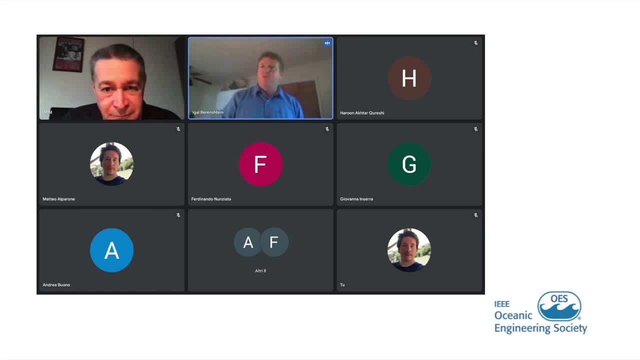 we take the currents from, we know where we take the winds from, we know how to plug everything in. so once that is done and there is, like, uh, active communication between the different components, to do another spill, like to model another spill, will be much faster and much- uh, you know, much- more. 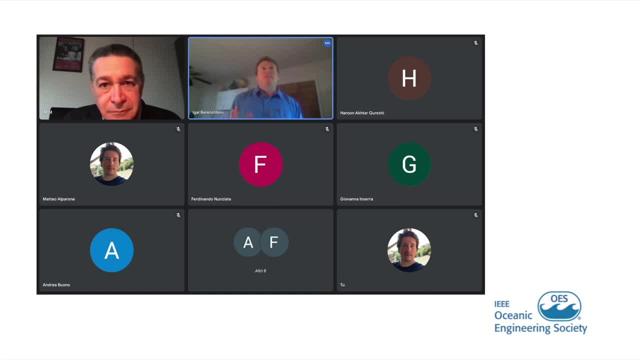 fluent, but but this type of of approach has to be um taken in advance. we don't need to wait for an event to occur. we we can talk between us, the, the remote sensing people, the, the oceanographer, the, the, the ecologists, and and create a framework that works before there is a spill and then once there is a. 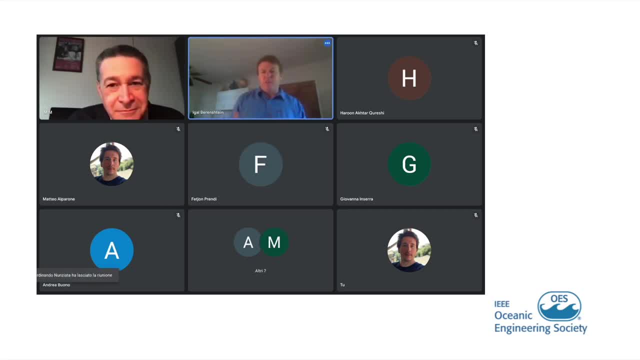 spill. we can do that uh quickly and easily and provide information from for the uh, for the management, for the decision makers, and i mean they can use it. they may use it and they may not use it, that's fine, but at least as scientists we're doing the best we can to help if the you know, if 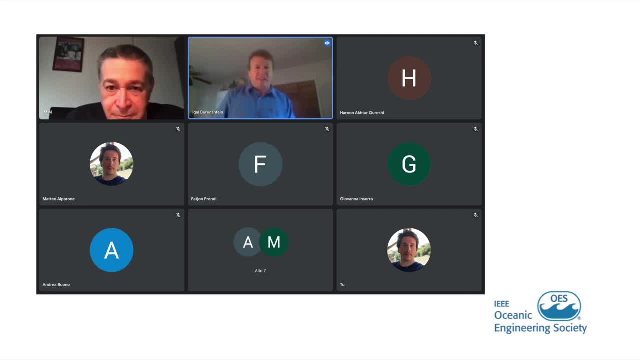 there's no use in that information. at least we provided it so. so i think that's kind of my approach, but at least for there is a um, there is a, a channel of communication between, for example, myself and people in israel that uh work on on spills, and i think that's.